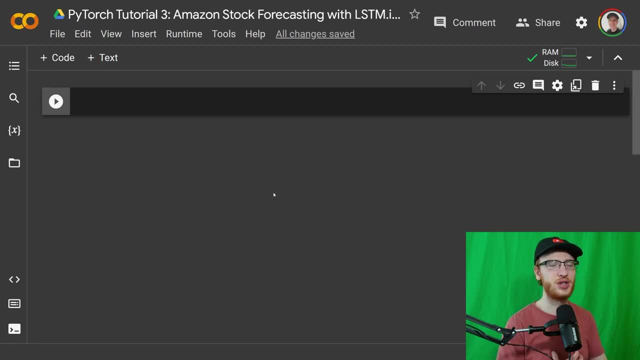 Hey guys, how's it going? My name is Greg Hogg and in this video, I'm going to show you how to do LSTM stock forecasting in PyTorch. It's a really important skill and a great way to improve your PyTorch knowledge. so don't click away. It's going to be a really helpful video I'm going to explain. 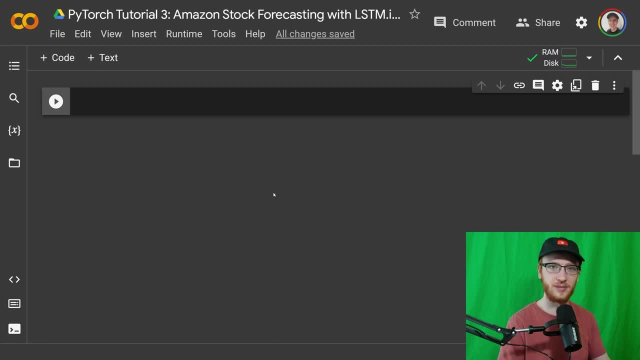 every step of the way. super simple. so let's get started Now. firstly, I'm just going to get a couple imports out of the way. Really standard stuff: pandas, numpy and matplotlib for graphing and data frame usage, and Torch is PyTorch and we're getting their neural network module for. 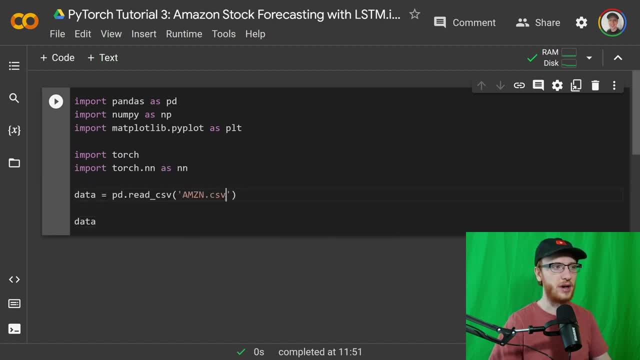 later Then we're going to load up our data as a pandas data frame. Mine is called amazoncsv. It's just all of Amazon's daily stock history. You can get that, either your own, from Yahoo's website or, if you want, the exact same copy I'm using, which is what I recommend you can find. 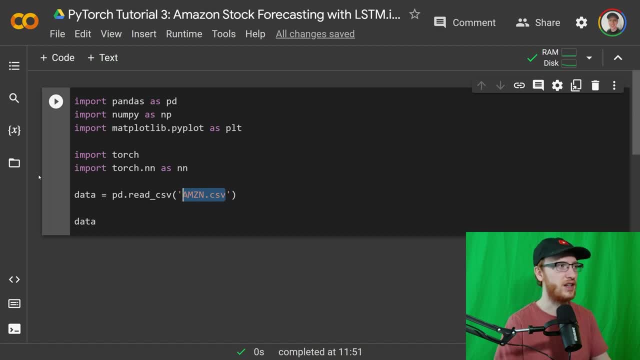 that in the video description. You can download that from my Google Drive and then, if you're using Colab, you can go and upload it over here, like I did. Okay, let's look at our data set. So we open our data frame. 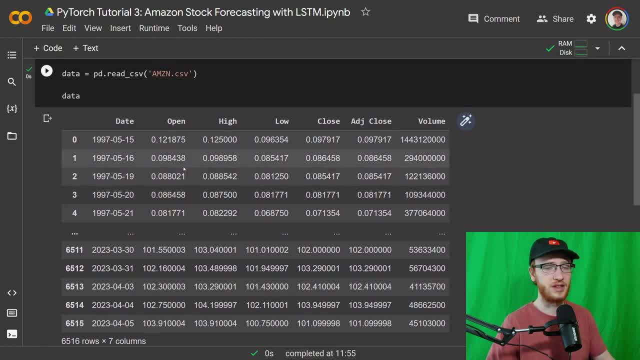 6,516 rows by 7 columns. This is daily stock history of Amazon. We have the open value, the highest value for that day, the lowest value for that day, the closing value, which is what we generally care about, and there's an adjusting close and the volumes of shares traded. We don't 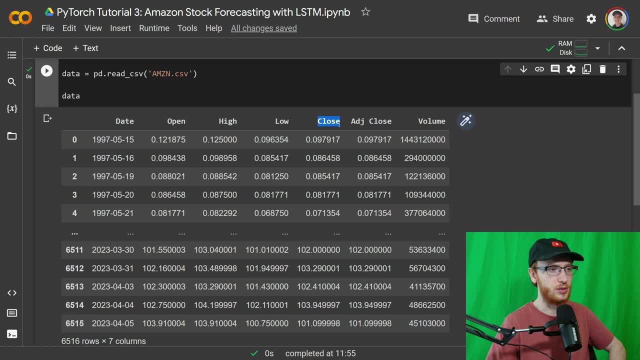 care about almost all of this. basically, We're just going to look at the close column Now. something that might look a little funny to you is: why is Amazon worth? like what is this? 9 cents back in 97? No, Okay, so they weren't worth 9.. 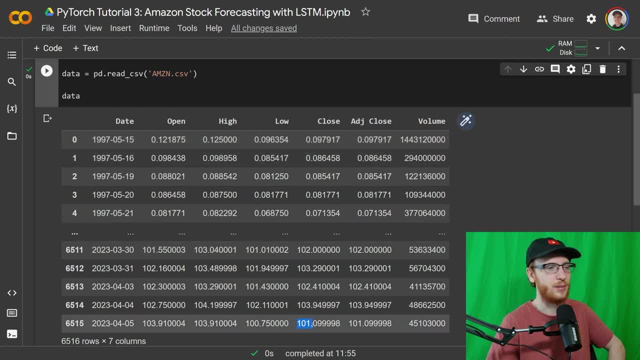 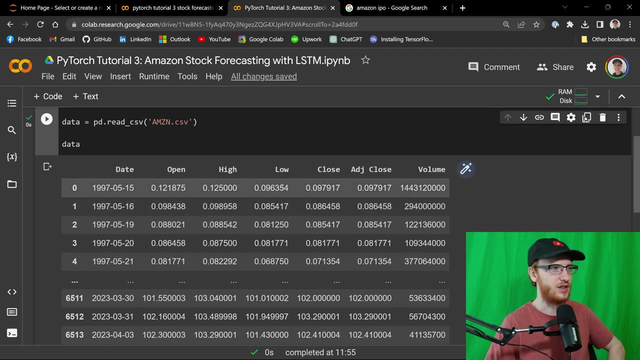 cents. It's that basically to say that this number is that much bigger than this number. Well, you have to kind of do a bit of an adjustment on what it was before, Because if you actually go and look up Amazon's IPO value for $18 per share, okay, so we don't see any history of that, we don't see $18. 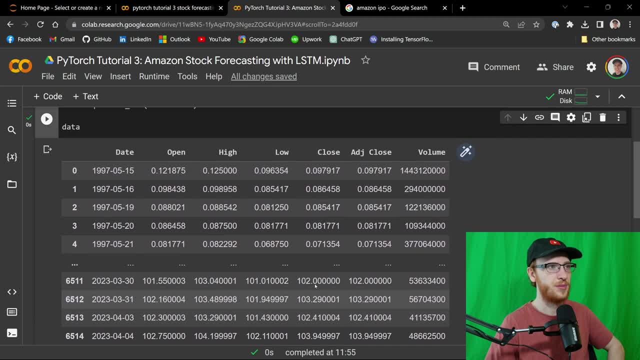 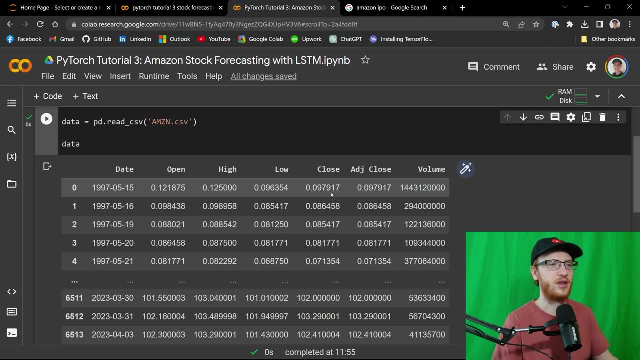 because this is $101 at the very end of this. So basically they do an adjustment, because what stocks end up doing is they basically do this split thing every now and then they'll say like, hey, let's just divide our stock value by two. and so, since it was, $200. now it's worth $100, and that's just because they want to keep it kind of standard with other companies. you don't want it to look like Apple's worth 10 times as much as Google, if it's actually not. if you didn't understand that, don't worry. I recommend you do some stock analysis, because it's. 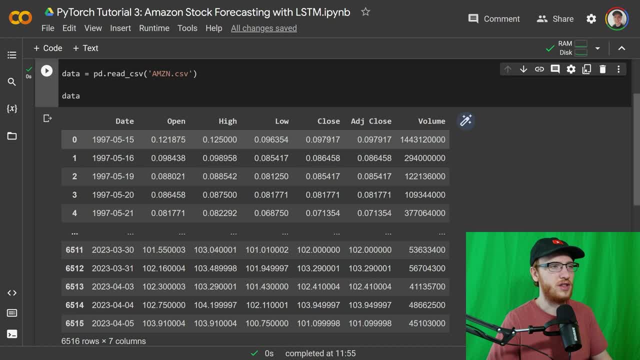 actually very interesting for your own daily life. but that's basically. the deal is that they did a bit of a transformation here so that this value is actually representative of it's that much more than it was before. don't worry about that anymore, okay, but as I said, we only really care about the 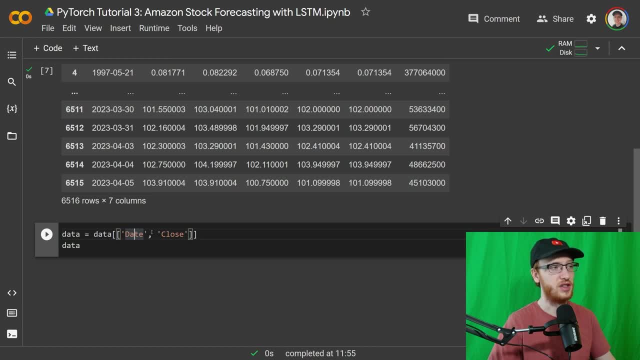 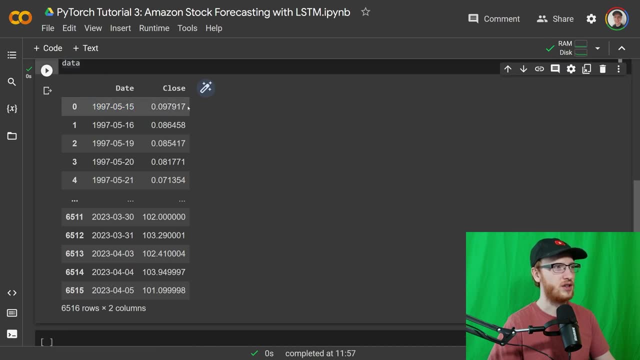 closing value. so this is just going to make that data frame only have, well, the date as well and the closing value. so a subset here and now we have the date when that was and the closing value of the stock for that date. this is what we're going to be forecasting now. remember on PyTorch by 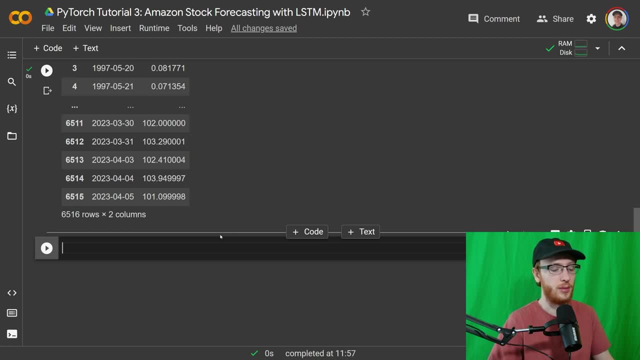 default, it's going to use CPU, but if you want to use a GPU, you can use a CPU and you can use a GPU and you can use a GPU and you can use a GPU and you can, which you probably do. you should do something like this: where a device is q to zero, if torch. 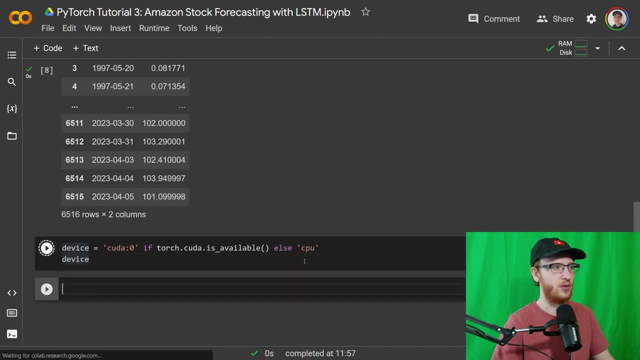 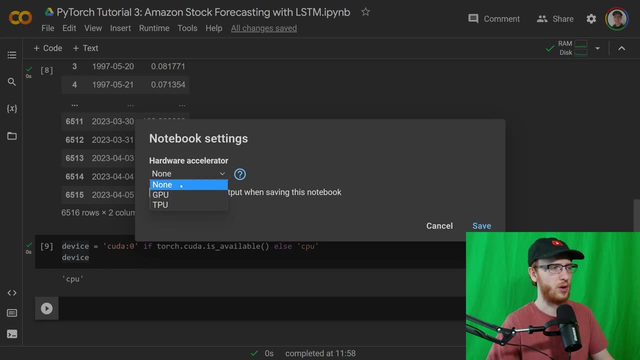 dot q is available. Otherwise, you want CPU And right now, if we output device, well, it just depends on what runtime I'm running. Right now I don't have a GPU, So it said CPU Later when we. 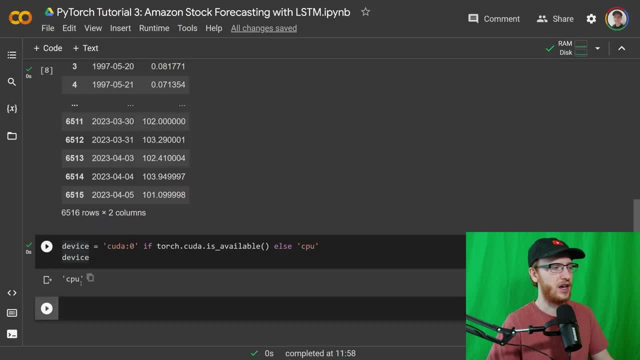 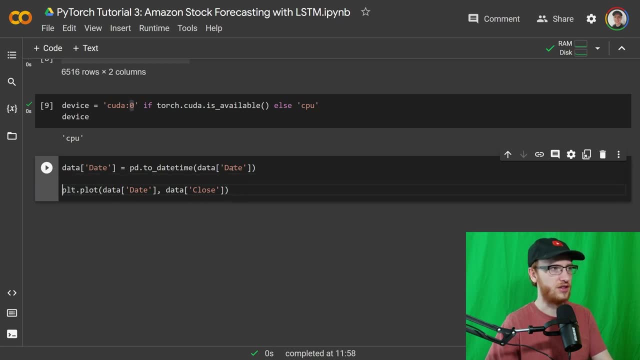 get to the training part, I will restart it and switch to a GPU And we'll see that that switches to q, to zero. Okay, now we're going to do some simple transformations. we're going to make the date column a pandas date type, So that's pretty simple. And then we plot the date and the closing. 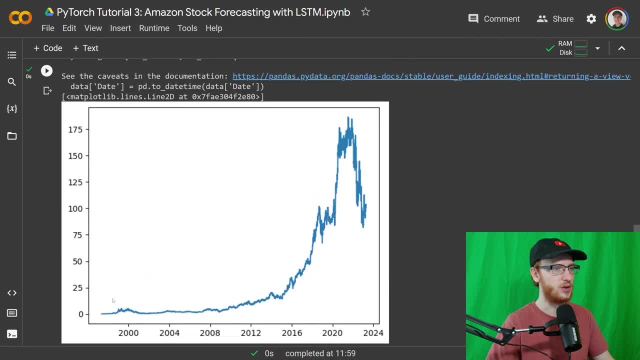 value. So over time we should see here it goes boom. Okay, so, as you can see from before like this: it's not that Amazon was worth like $1 or 18 cents or whatever it was at this point, It's just 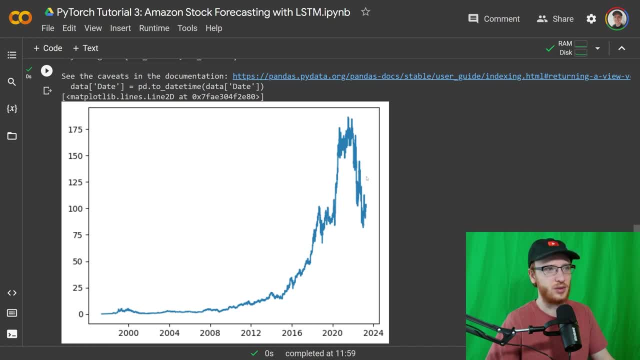 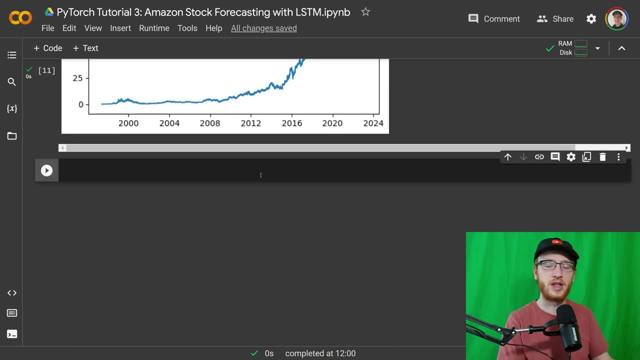 a transformation so that it shows that it actually grew this much And then it went lower. here Again, don't worry about that too much. Now I want to set up the data frame in a way that's close to how the model is going to take the input and train off of it. So basically, an LSTM is looking at history. 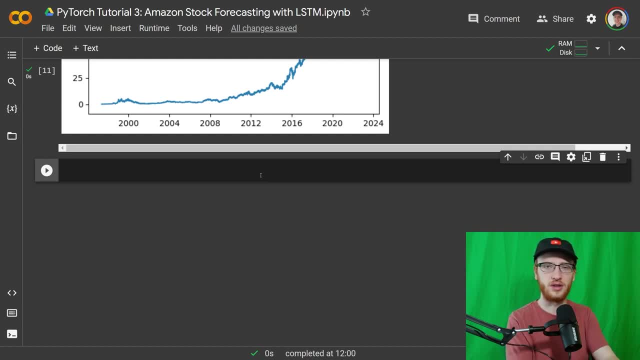 So for one particular date it wants to know what the closing value was for that date and the day before that and the day before that. we can do that with this massive block here, And I'm going to explain how it works shortly. But don't worry about the code here, I'm just going to run that. 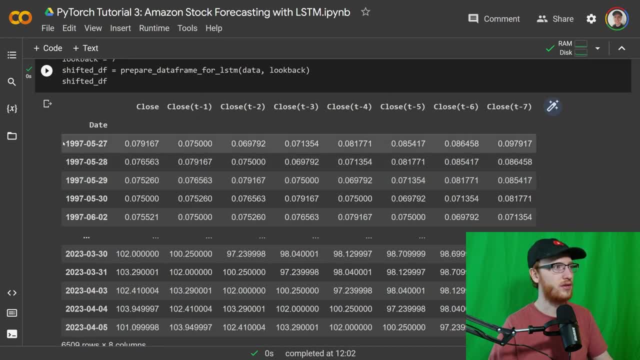 and check. take a look at this data frame that we produced. we have for any particular date. here we have the closing value for that date, So it's just close. that's the same value. then we have t minus one, which means the previous day. So on the 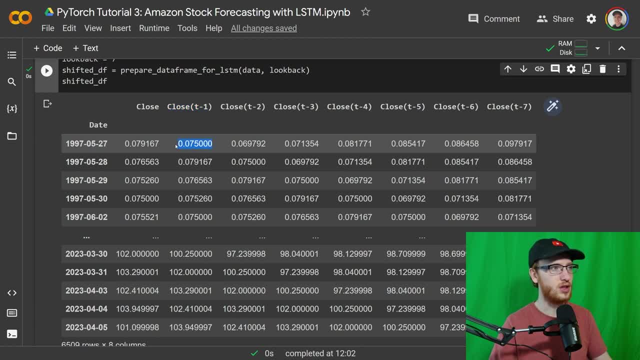 previous day, which would be the 26th. this was the closing value, And for two minus two, it would be the 25th. This was the closing value all the way up to a week beforehand. t minus seven. we have that. 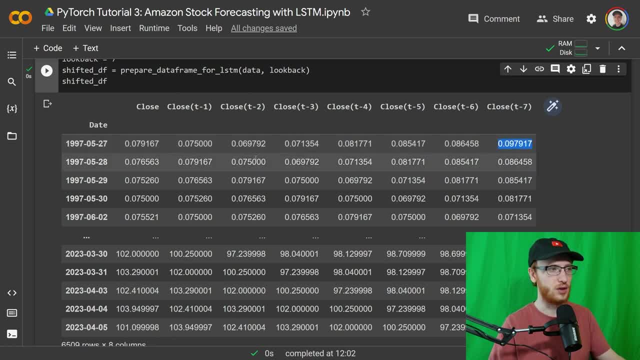 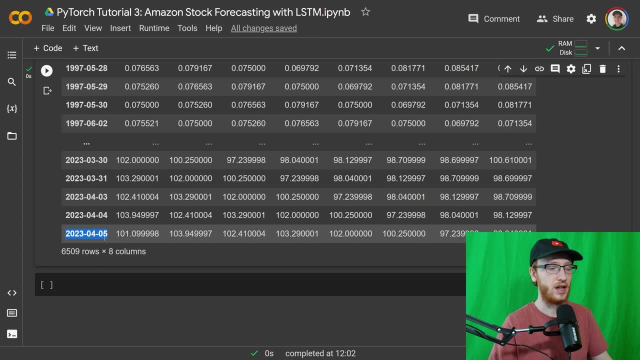 would be on the 20th. This was the closing value, And this goes all the way from this. you know original value here- all the way up to this, which is the end date that I have downloaded, And so it's the same deal. This is t minus one. 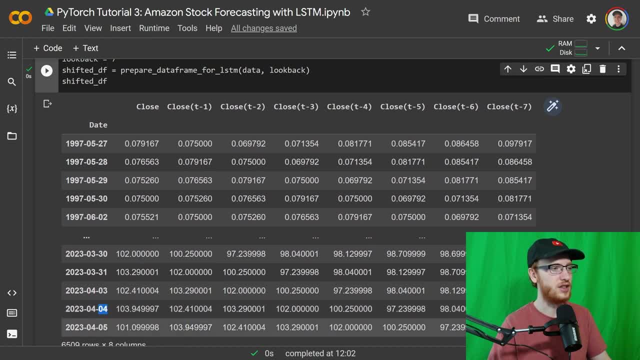 or so. this is the value for the fourth, So you should actually see it here: 103.949. And nine: that's that value there. Okay, so it should be in this diagonal format here, where, if this is t minus two here, well, t minus two, we go minus two, And there you go. 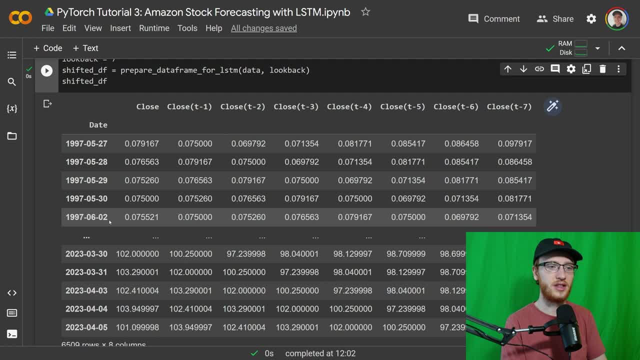 the same value. That's the closing. Now, the reason our model likes this is because in here we have an input matrix x and an output vector y. Here is our input matrix x. it's t minus one, all the way all of this stuff. And then here is our output vector. Why is that the case? Well, 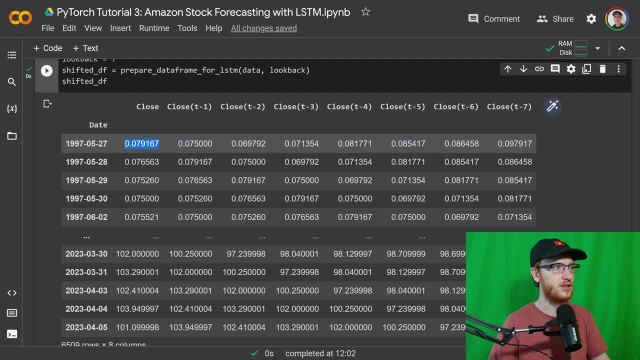 this vector is what we would use to predict this, because we're looking at t minus one, t minus two. we're looking at the last week of history to try and predict what this would be. Now, of course, we know what this is because this already happened in the past. 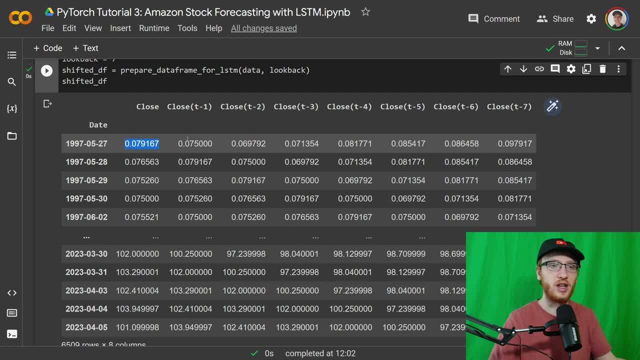 But that's what you use. you use data to try and inform and train the model that, hey, this is our last week And this is what this next day turned out to be. Now for this date, this is what the last week of history was And this is the date we're predicting on all the way up until our very 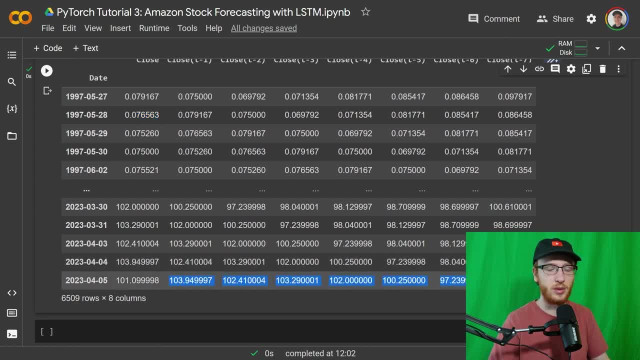 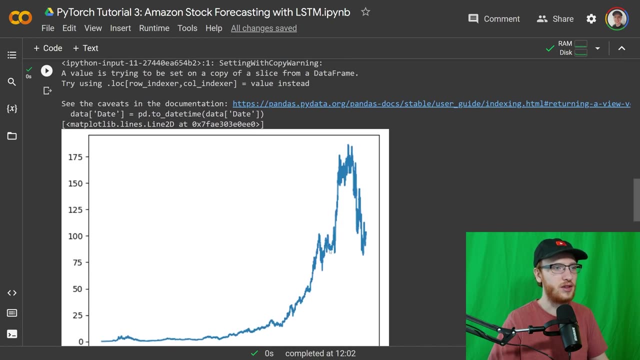 last data point we have, this is the last week that we were training on. this was the last week of history, And then we're trying to use that to show the model. hey, this is what it was then. And what's really informative is because look at the graph, like in general, if you give it, say, a week, 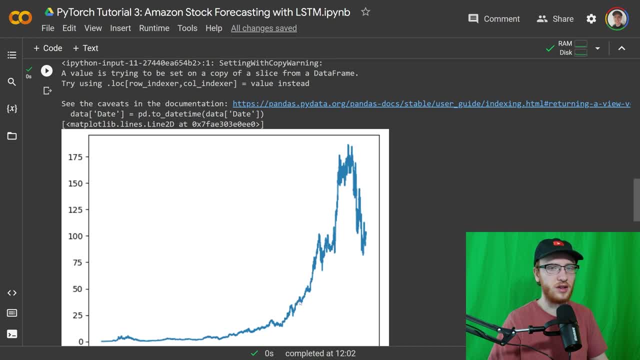 of history it's gonna see like: okay, well, clearly in this week here this was going up, So of course the model is probably going to predict that it would go up, or here in this week here clearly there was parts where it was going down, And so the model is probably going to predict that. 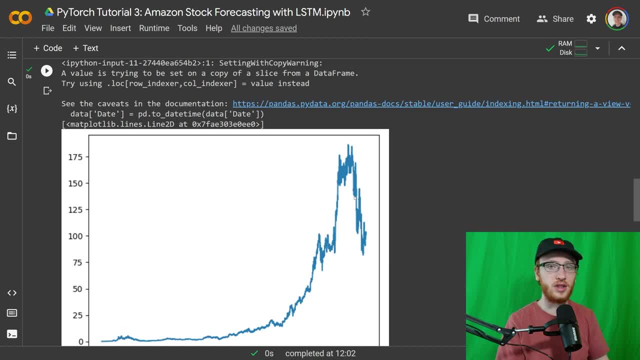 would go down. We're trying to learn the sequential pattern. This is why we're using a sequential based model in RNN, Because it keeps checking: Okay, the price went down again. price went down, it down again. price of it down again. i'm probably going to predict that the price is going to go. 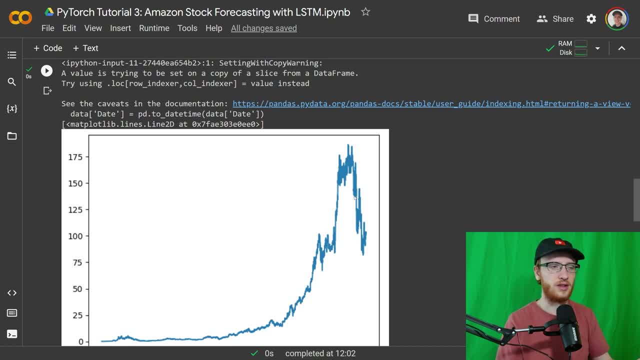 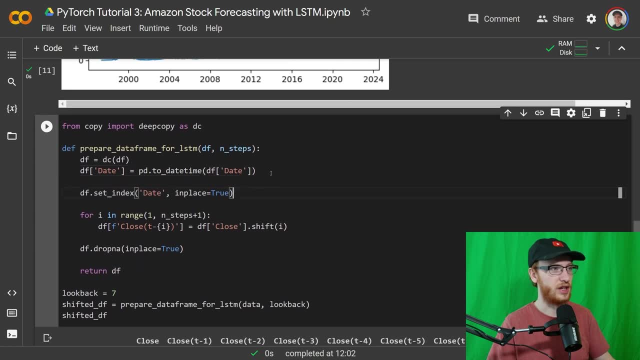 down again, or if it was going up the recurrent network updates: it's going up, it's going up, it's going up. okay, i'm going to predict that it goes up. now i don't want to focus too much on the code here, and actually i realized that we're not going to need this duplicate line again. basically this: 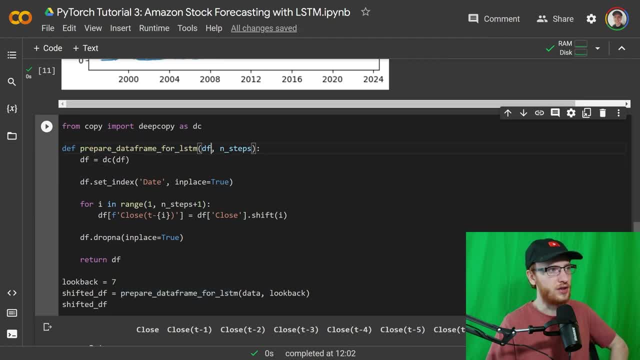 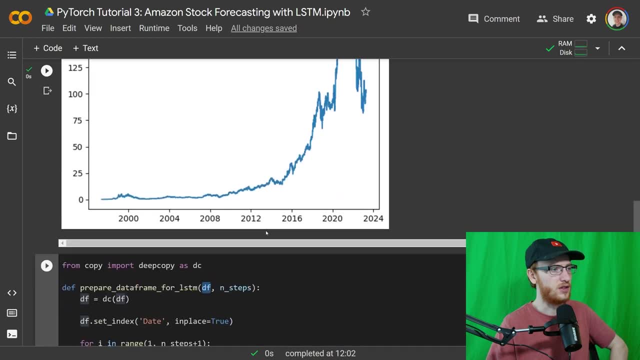 function is it's going to prepare a data frame for an lstm, where it takes a data frame like the one we had above. it just has the date and the closing value, so a simple data frame. it's going to take that and then a number of steps or basically a look back window. we passed seven. 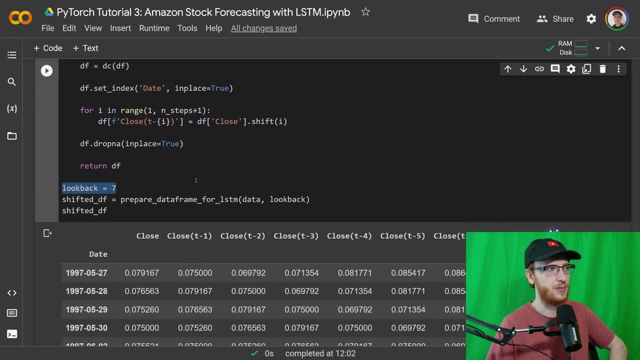 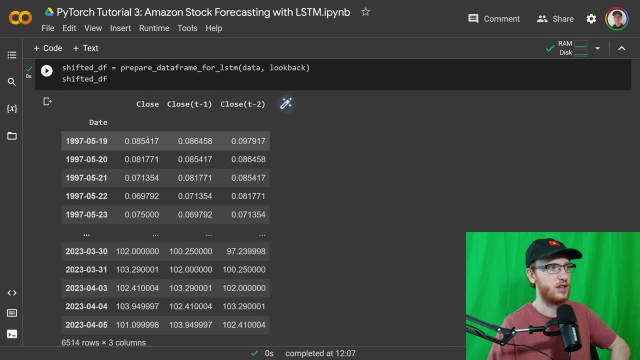 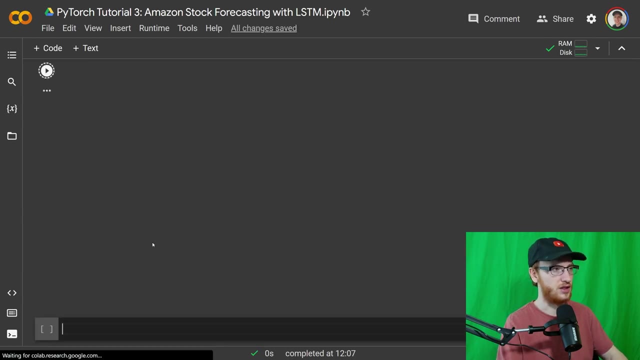 hence we saw we got t minus one up to t minus seven. if you instead passed, look back is say two and we run that again, we should see we have very similar things. we have the closing value for that date, but then only up until t minus two. so i'm going to stick with seven for this example, i think. 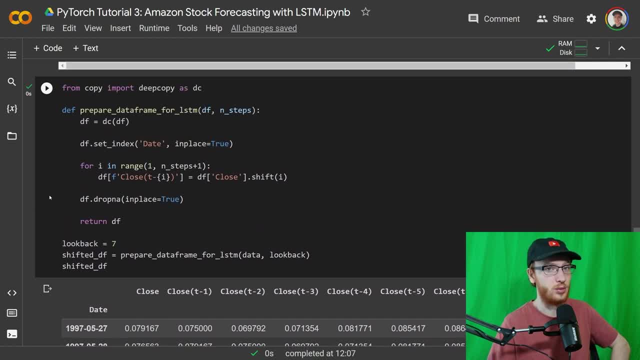 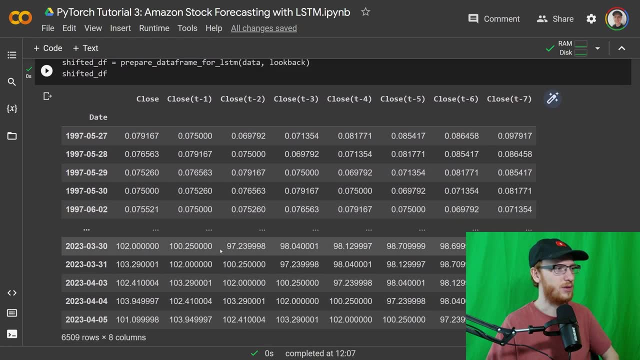 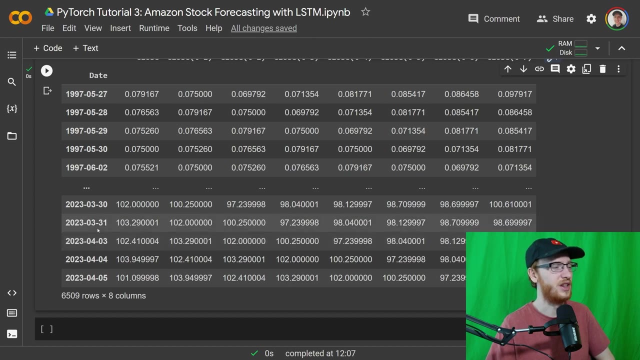 it's easy to explain and it just makes sense for the model to have a week of information. don't worry too much about you the fact that stocks aren't running on the on weekends. this actually does prepare for that. as you can see, there's a jump between. well, that's april fool's day, so that'd be kind of funny. but 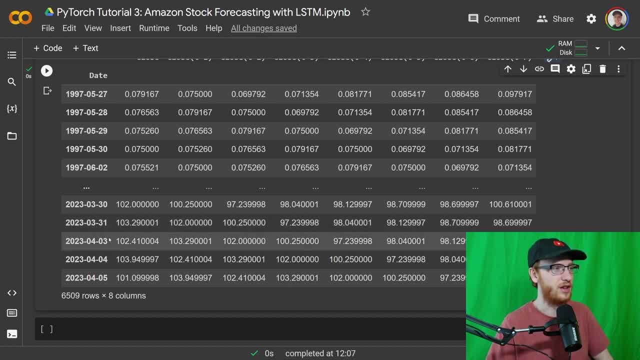 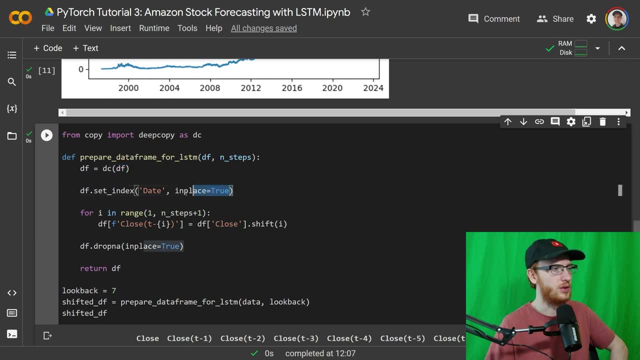 there is no april 1st or april 2nd there, because that would have been a weekend, but yeah, basically, this function is going to make a deep copy of the data frame and it's going to set the index of that to date in place and then it's going to do a series of shifts and i don't want to show you how this. 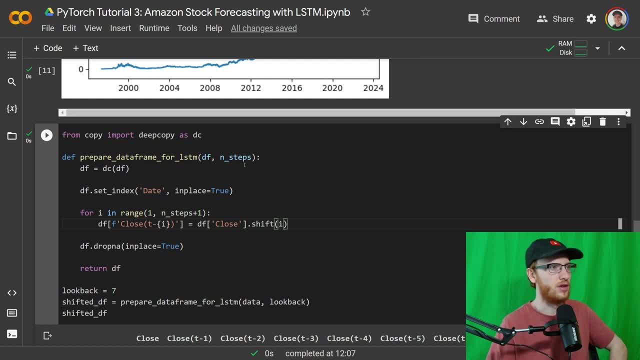 works, but it kind of keeps stepping where for the number of look back windows. it's going to keep shifting the data frame and it turns out that if you do it this many times, you step like this, then you're going to end up with this data frame here. i would just copy the code. you could dig it. 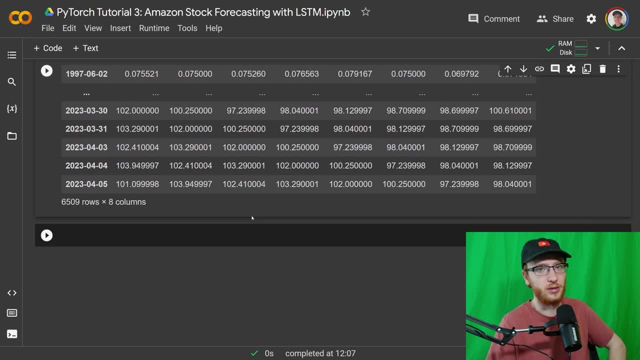 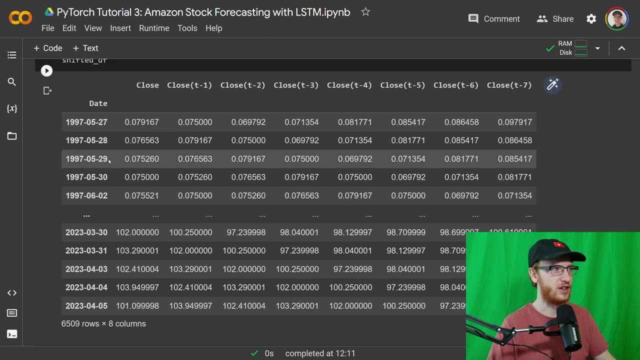 apart, if you really wanted to, would be a good practice for your brain, but not really necessary. so now that we have that data frame, i'm just going to convert it to numpy. it's the same thing, but to numpy, and it's not going to take the date column, it's just going to have this as the first column. 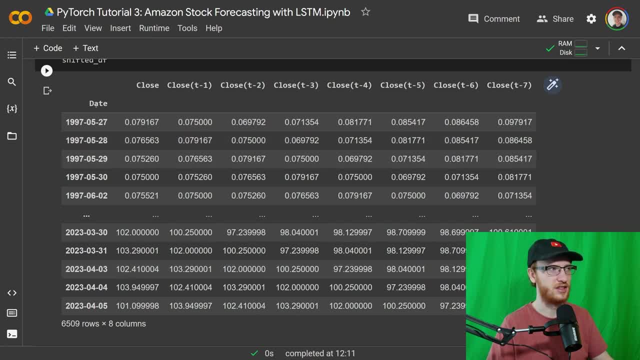 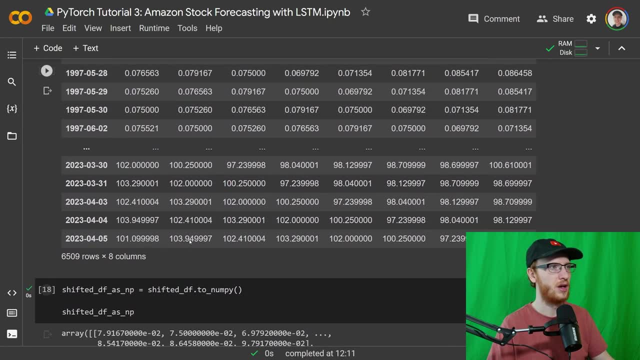 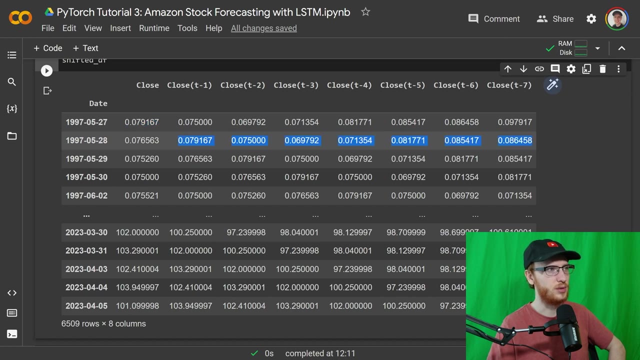 because this is set as the index. right now, you can kind of see that this is lower because it's not part of the data. so this is our massive matrix, which is shifted df as numpy. now, remember that, since this example is going to predict this and same thing, this is going to predict this, basically. 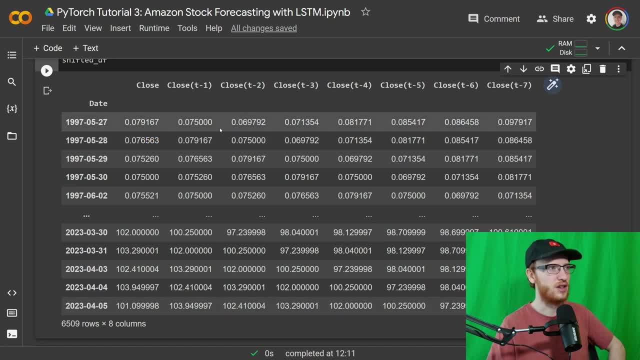 this is our vector of outputs y and this is our matrix of inputs x, so that they line up, so that each of these examples is using to predict this, and we're also going to take a subset of this and make it the train and take the other subset and make it the test. we'll just make the train. 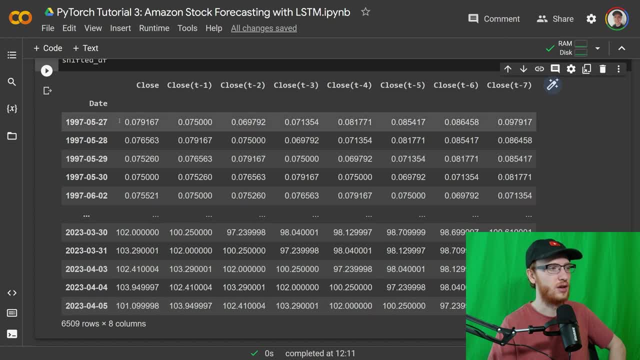 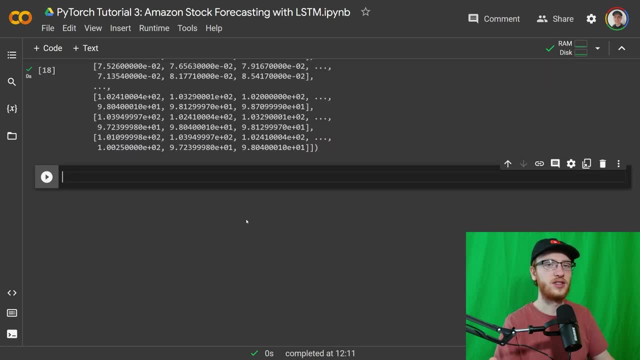 some first portion like the first 90 or so percent going up like this, and then the last 10 percent rows are going to be for the test. now, before we worry about x and y and train and test, we're just going to run a scaler on all the data. so we'll do a sklearnpreprocessing min max scaler. 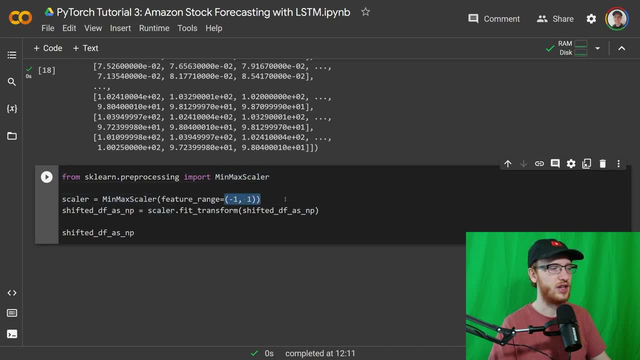 and we're going to run a scaler on all the data. so we'll do a sklearnpreprocessing min max scaler and we'll get the scaler. is that with the feature range of negative one to one, we will overwrite our matrix that we have above and just run the transform and fit it on that matrix and we 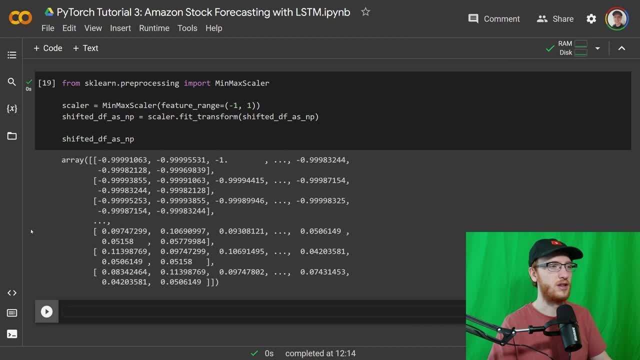 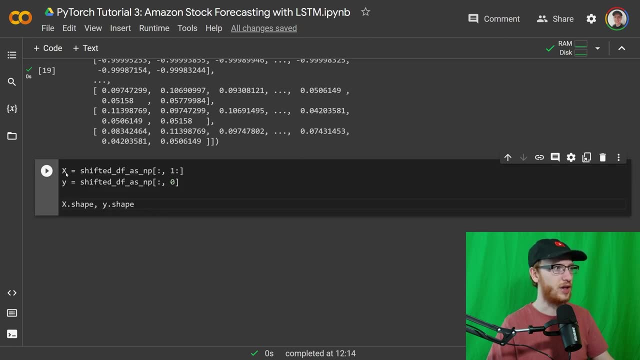 should see something that looks very similar to the above, except the features are going to be all between negative, one and one. okay, now that our data is scaled, we're going to make this x and y, so we have x, our matrix, x is that matrix above the scaled one, all the rows, but then just the. 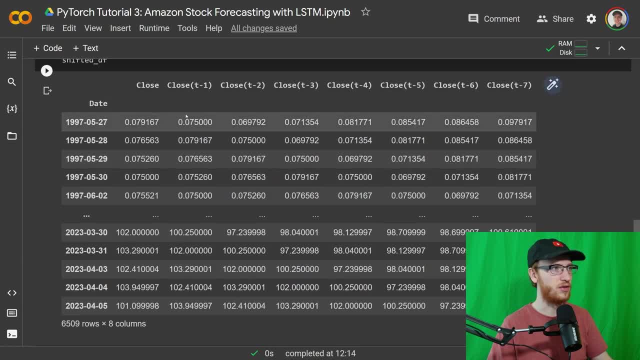 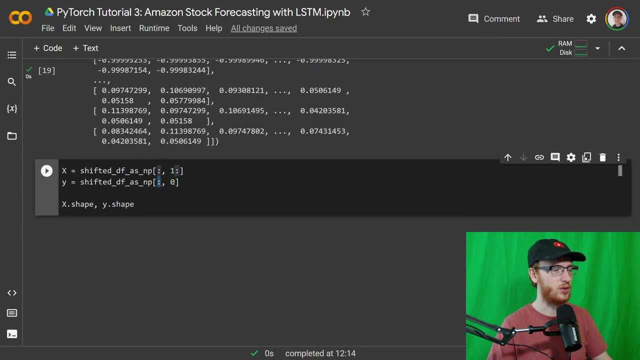 first column onward, because we're going to have a matrix x and we're going to have a matrix y, because that's this piece here, the first column onward, and then all of the rows, so that massive chunk there, and then y is just going to be all the rows, but the very first column, that's our. 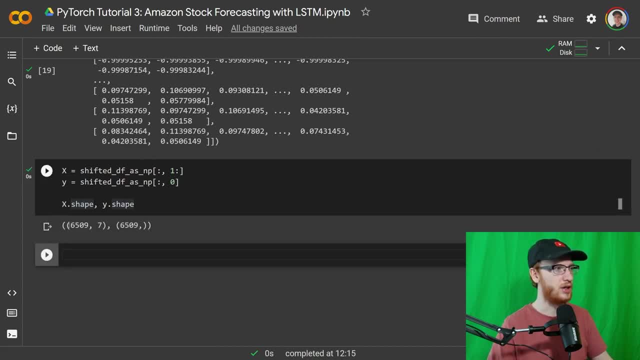 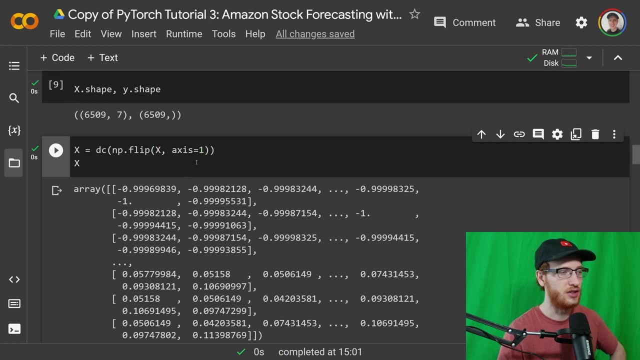 predictor and we have x dot shape and y dot shape. should be the same number of rows here, but for x we're going to have seven different features. sorry, this is greg from the future, fixing a mistake in my first recording at this spot you have to do. x is a deep copy of numpyflip. x on axis equals one. 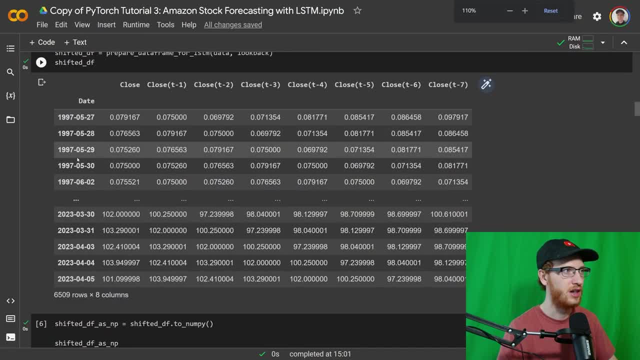 because basically this current data frame here it has t minus one to t minus seven, but for an lstm you would want it going t minus seven, t minus six up until t minus one, because it's kind of recurringly getting the more updated answer until it gets to the most close to the close value there. 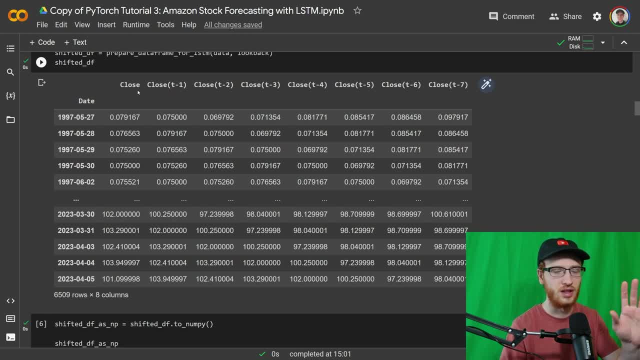 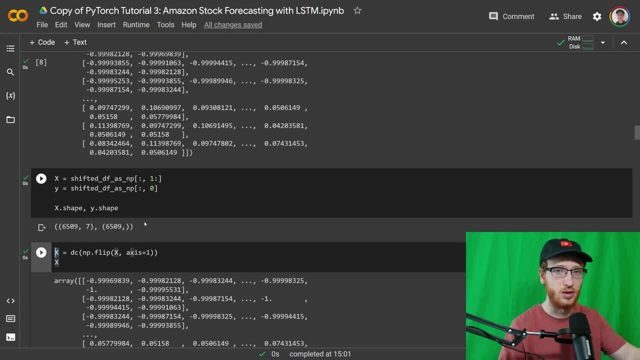 is so you would just want to flip that to kind of mirror this in the horizontal direction. so you're not going to see that in the upcoming cells because i forgot it in the first recording. but make sure you do that now. we're going to work on splitting this to train and test. we're just going to get a split index. 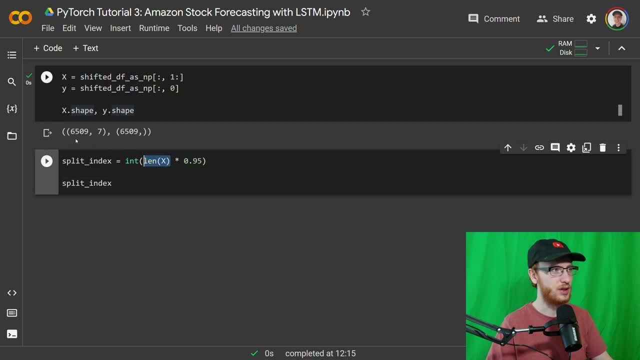 which should be the integer of the length of x, which should be 6509 times 0.95. so this means we're going to use the first 95 percent as train and the last five percent as test and our split index. so that's the row number at which we're splitting, basically, maybe off by one: 61, 83 now. 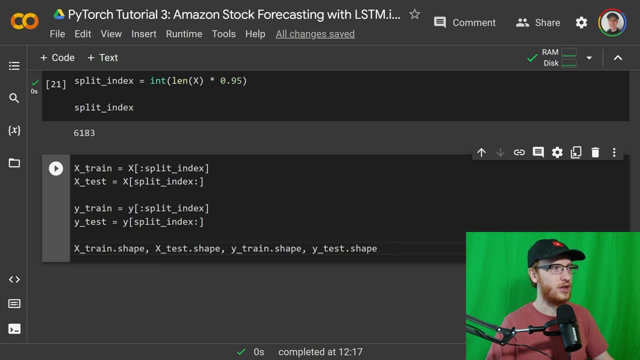 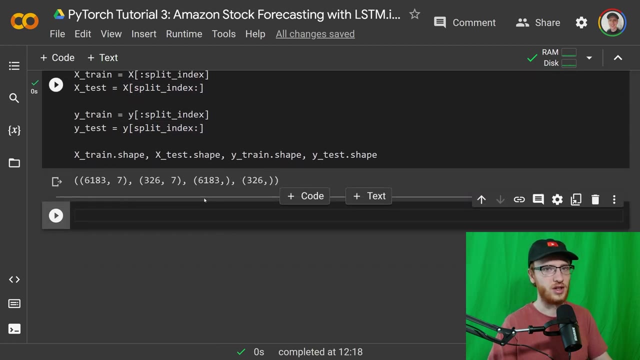 we're going to split x and y into train and test, so x is now becoming x train and x test and so x should be up until the split index and x test should be split index onward. very similar for y train and y test. and these are our shapes, which you should see, that these match up perfectly. 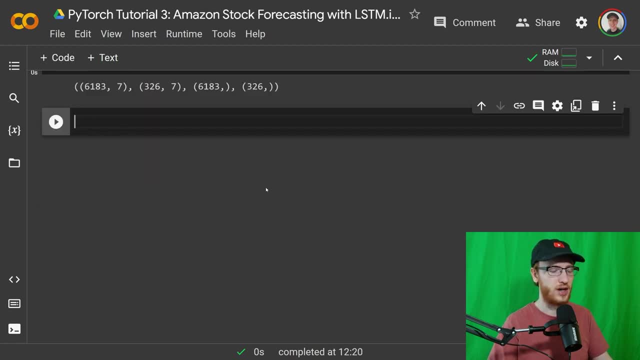 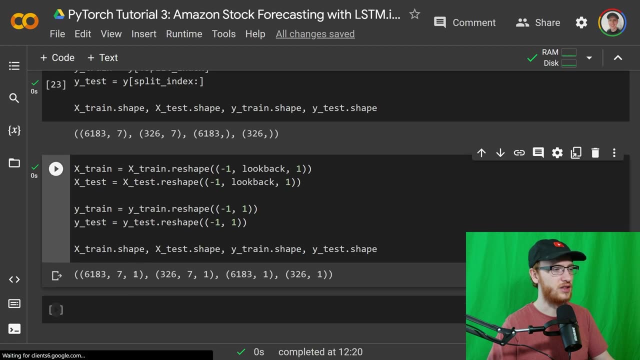 now it's a requirement for pi, torch, lstms to have an extra dimension at the end here. so we're going to do a bit of reshaping to all of these things, where the matrices are going to get another dimension at the end and the y vectors are also going to get another dimension as well. now, so far. 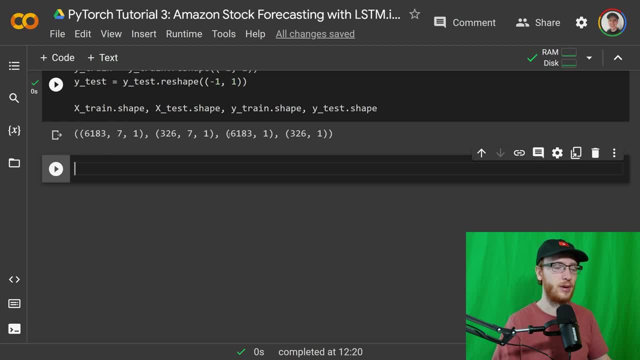 all of this is going to be a little bit more complex, but we're going to be able to do a little bit more of this stuff in numpy. but since we're using pi torch, it probably makes sense to wrap this stuff in pi torch tensors. so that is really all this does and makes sure that the values are floats. 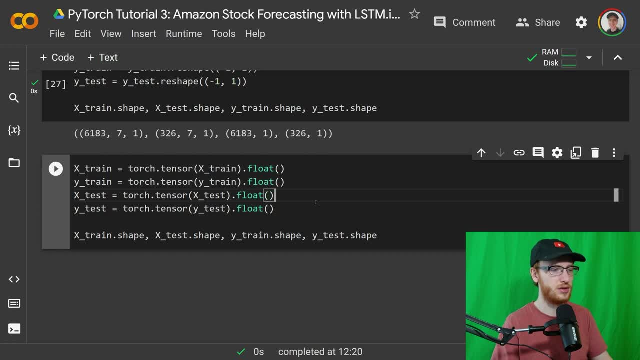 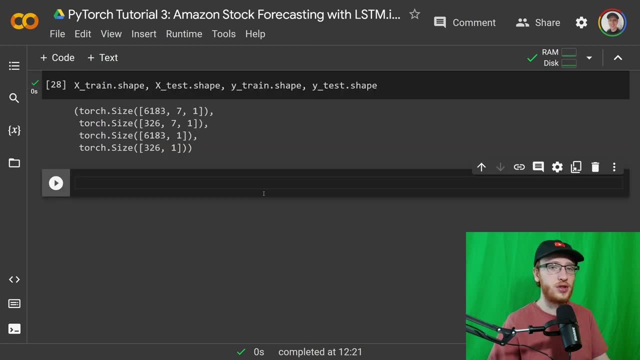 they're all making them tensors of themselves and then floats. we still should see the shape. but now we'll see pi torch shapes. they're going to look the same as above now. generally when training models in pi torch you use data sets rather than just raw tensors. so we're going to 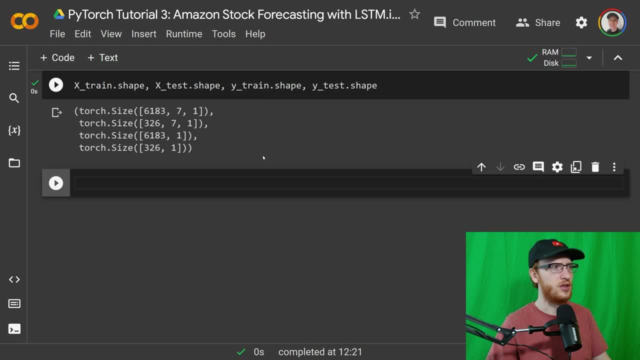 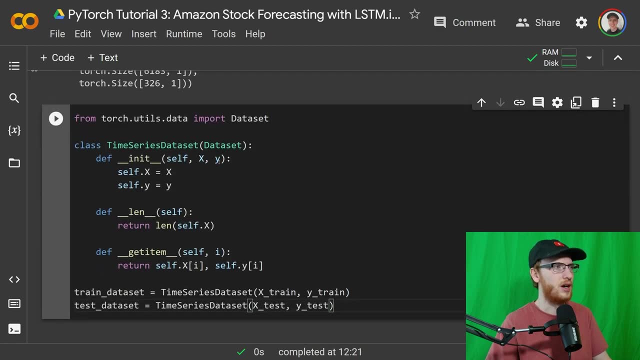 make that data set object. now it's really easy, but to do that you can't just like make data set of these, you have to make your own custom class, and it's really, really easy, but to do that we basically just make a data set and then we call it whatever we want as our class name, and then 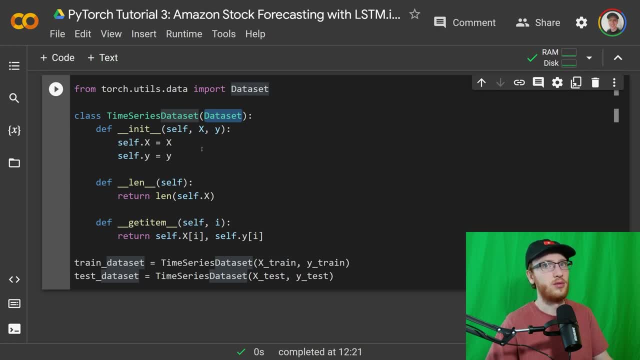 put data set in there and we have to specify three really simple things: a knit which takes a matrix x and an output vector y, and we're just going to store those in self with the same name. and then we get the length method where if you call len on this thing, it will return what it will. 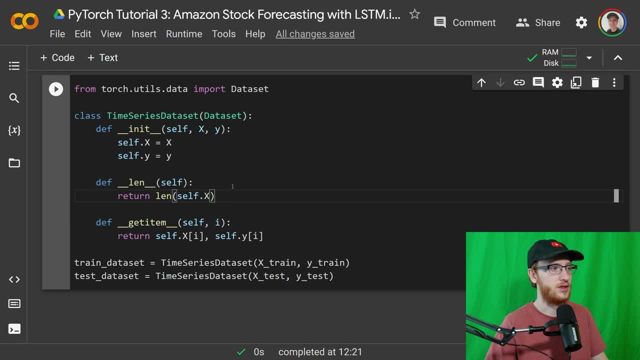 the length of x or also the length of y, that would be the same thing. And then get item, which is the, the square brackets thing, the indexing. that just gets x of the index and y of the index that you passed in there. really, really easy. it just returns that tuple And that. 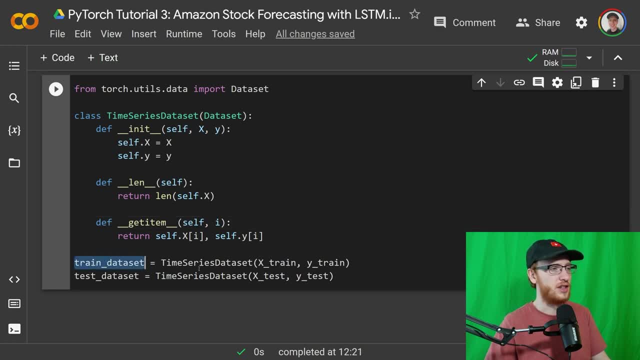 that's it. So from that we are going to make our train data set one of those passing in x train, y train and the test. with x test and y test we run that and I don't need to output anything because they're not really going to output much if you look at them, But just to take a look. 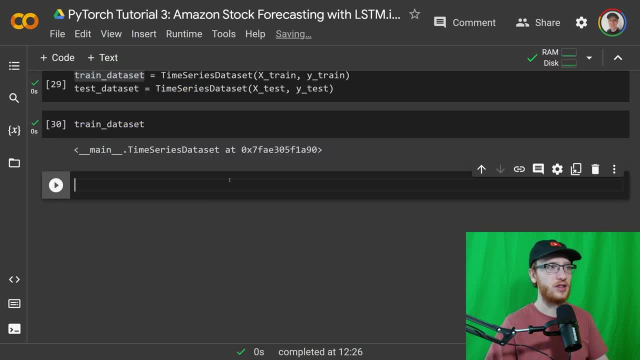 it's a data set. One more thing: we actually wrap these raw tensors not in just a data set, but we wrap the data sets and data loaders to get our batches. So we get our data loader here we'll specify the batch size is 16.. And we will get our train loader. is the data loader passing? 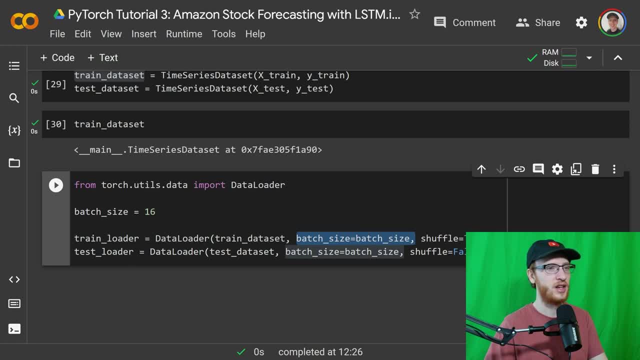 in that train data set with the batch size of what we specified, And we want to shuffle that every time and test. it's going to be the same thing, except shuffle is going to be false. we run that And here are our loaders. That's where we're going. 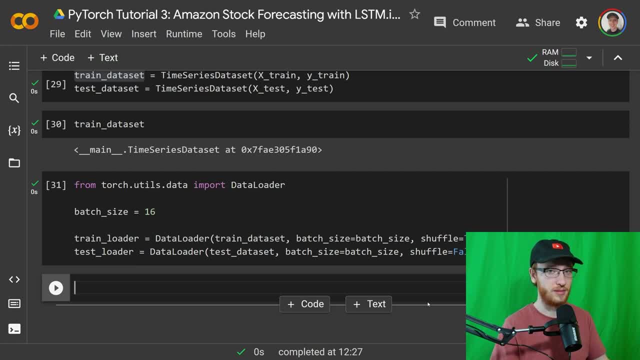 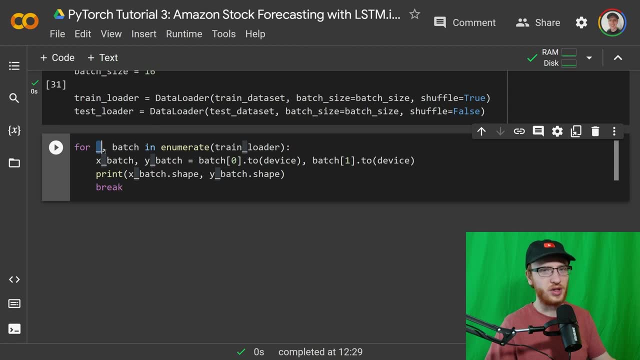 to use to iterate over, get batches and make updates to our model. Now, this next part isn't quite necessary, But for visualization it's quite helpful. We get for underscore later we'll keep track of something else. don't worry about that. We're basically just looping over. 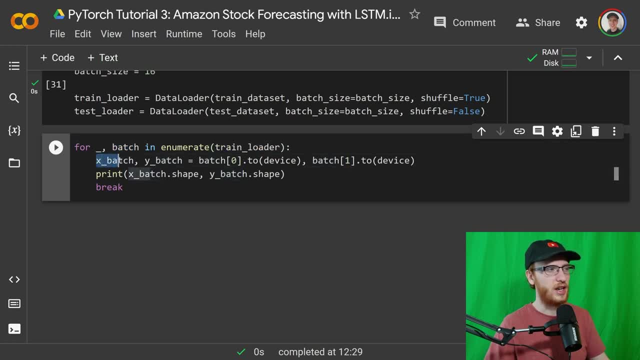 and getting a batch from the train loader And we get the x part of the batch and the y part of the batch. So what we're going to do is, well, the x batch will be batch sub zero and the y batch will be. 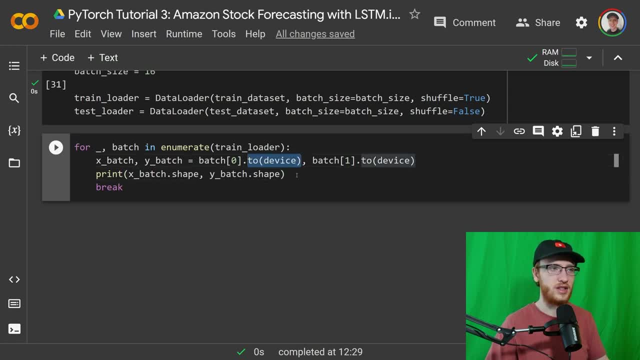 batch sub one, But we have to convert those or put those on the device that we're using. Later, when we make the model, we will make sure that the the model goes to that device as well. So we put it to either the CPU or the GPU And then we're just going to look at the x batch shape and the y. 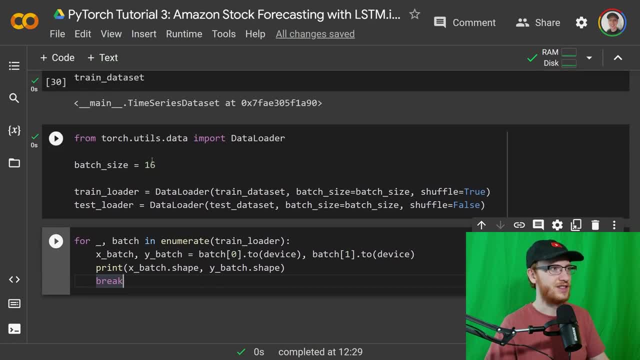 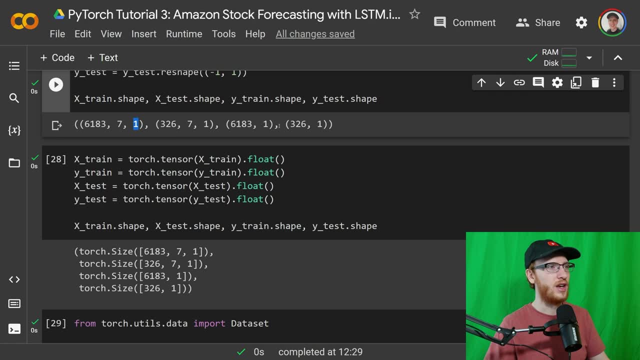 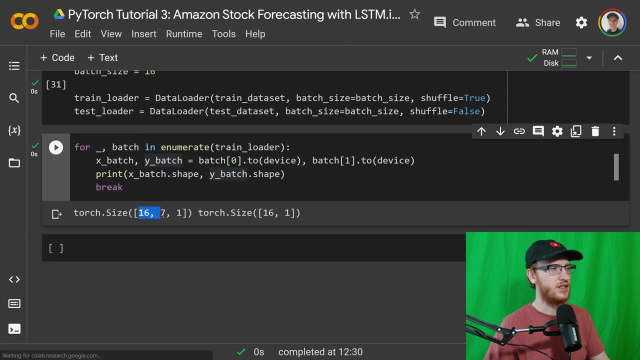 batch shape. What are we expecting? Well, since the batch size is 16.. And what are we looking at for the inputs? Well, the inputs are: the x should be seven by one And the outputs should just be one. Okay, so we are going to see that we have our size of 16 by seven. 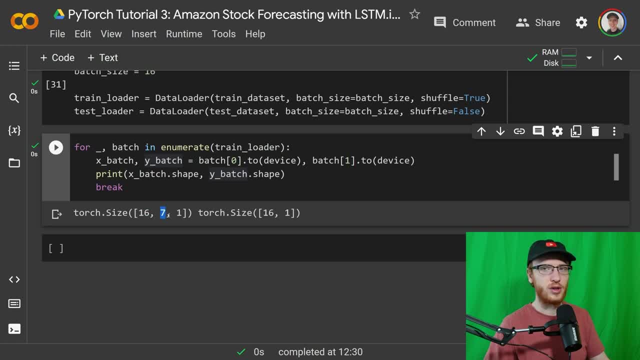 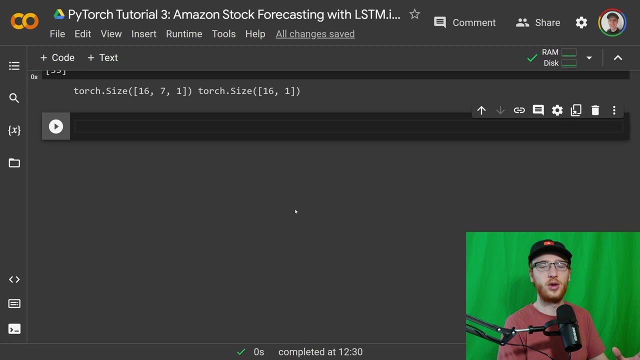 by one. we have 16 examples where we have the seven look back window and then just that extra one there, And then for each of those look back windows we have our predicted output, which is just one value. Here's where we create our model. In a moment I'm going to paste a ton of code on. 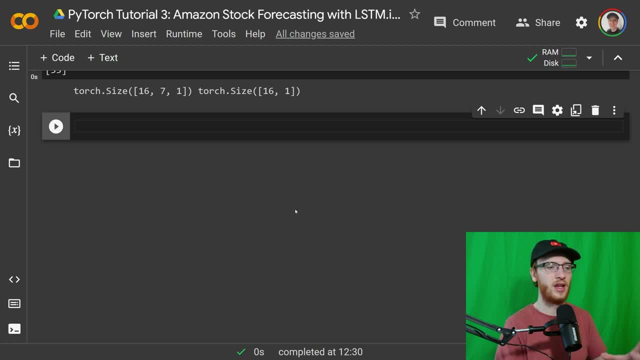 the screen, So don't feel bombarded. I'm going to explain it every step of the way. Let's be honest, this is confusing. It's a confusing model, And LSTM and pytorch are just more annoying than they are in TensorFlow. Of course, like most trade offs here with pytorch and 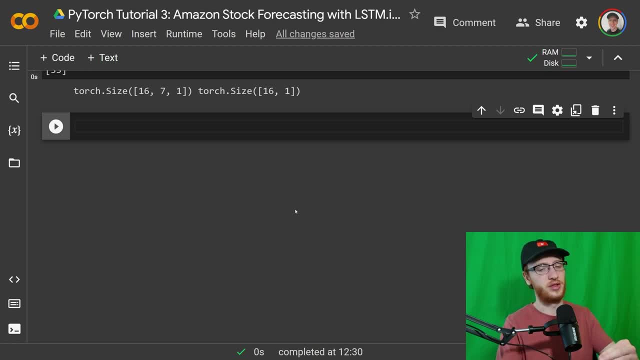 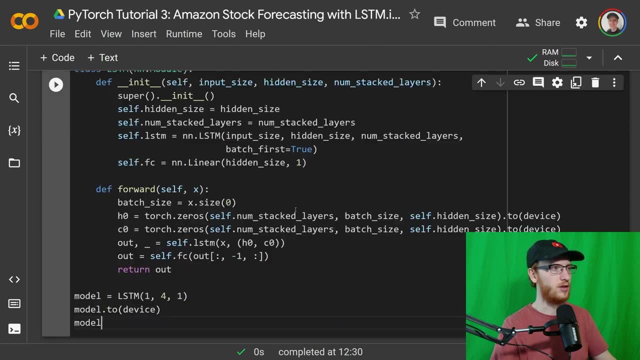 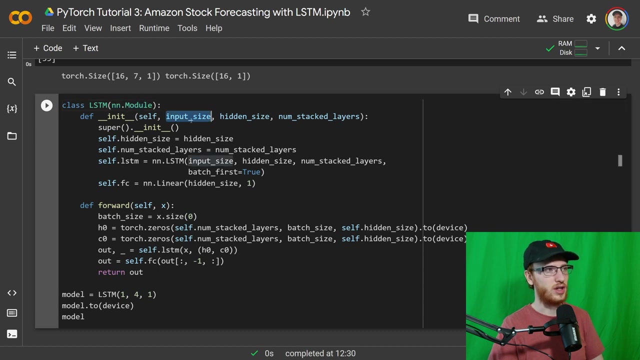 TensorFlow. TensorFlow is a little easier for beginners, But pytorch is a little more flexible for people really in the field. Here it's going to look pretty confusing, But let me try my best. So here's our code. we have a class LSTM neural network module. it's going to take in the input. 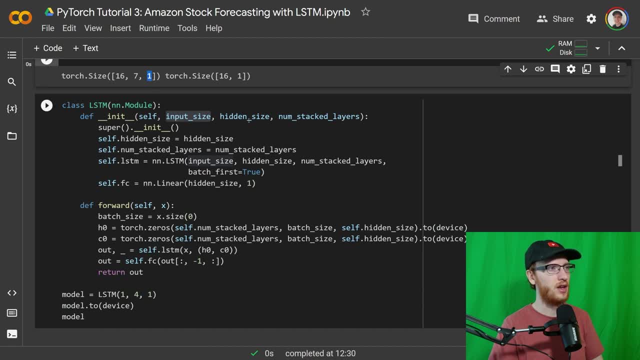 size, which is our number of features. We'll pass that a one hidden size, which is however much, however dimension we want to be in the middle, there could be 12432, the same type of thing in a linear layer and number of stacked. 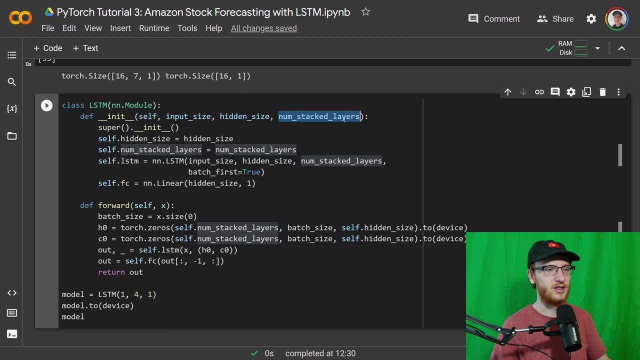 layers, which is basically you can stack LSTMs Because as they recurrently run through themselves, they're going to produce a sequence themselves. they'll produce a sequence of hidden layers, And so you can stack these things if you want. If that didn't make sense, I would check out, Andrew. 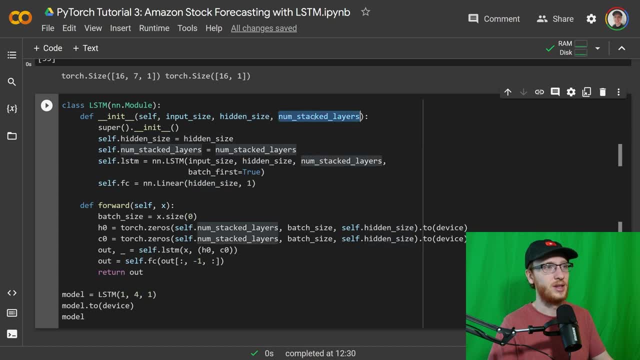 Inks courses If you want to hear about that. Otherwise, just take it as the more of these things that you have, the more complexity that your model would have. So we're going to do our standard super init. we'll get to the hidden size. 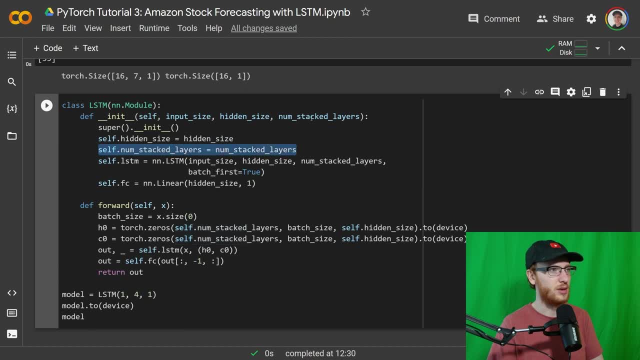 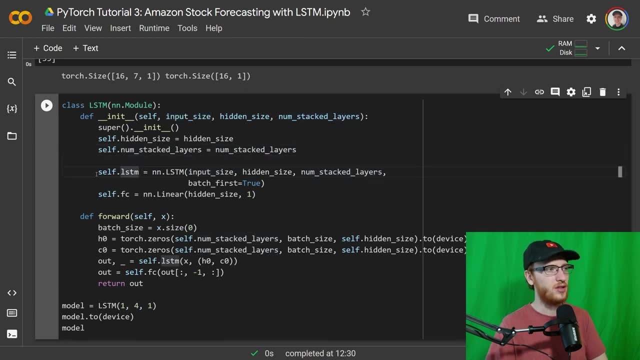 is the hidden size. our self numstacked layers is the numstacked layers that we don't need to keep track of the input size, because it's just where we create our LSTM part. So the LSTM part of the model is going to take an input size which, again, is just the number of features we're looking at. 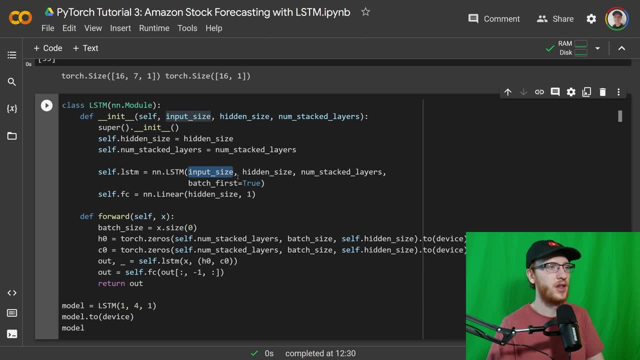 it's just going to be one thing, because we're just looking at the closing value, the hidden size, whatever we defined for that, we're actually going to end up passing four of those And number of stacked layers. Again, I'm just going to give that one because it turns out. 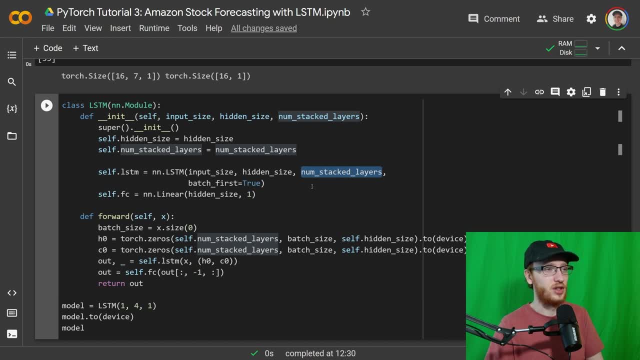 that this model is going to overfit pretty well anyway. So we're just going to use one of those And batch first is true, which means that in some later pieces you'll see that it returns the batch as the first dimension. Finally, after your LSTM, it does the recurrent part for taking 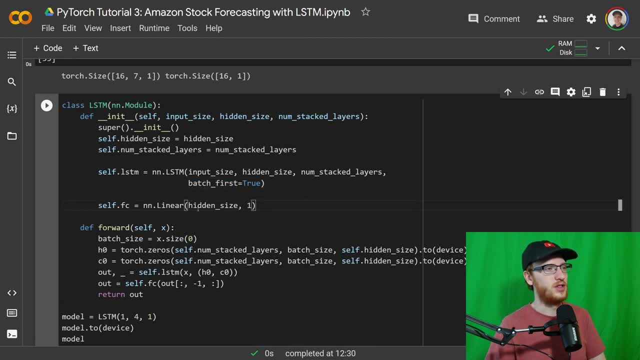 in the sequence. you would want a fully connected layer which is going to map from your hidden size, whatever that hidden layer was- to just one, because at the end of the model you need that to predict just your final closing value. So that's. 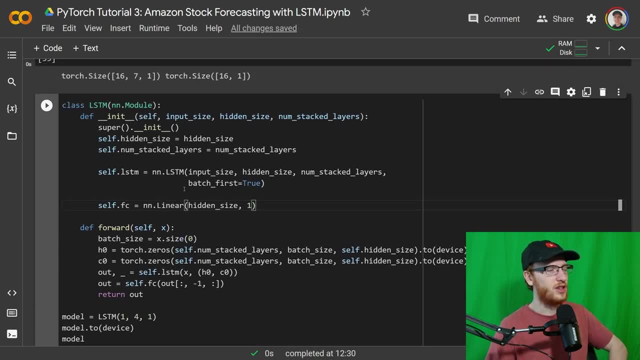 why that's a one. Okay, and then what your forward function does is going to look extra confusing, if that wasn't already confusing enough. we have the batch size, which is x, dot size sub zero. So you have to kind of dynamically get this size from the input. that's important. And then we have h, zero. 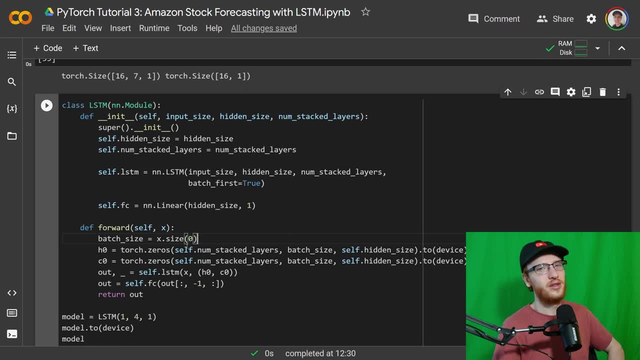 and c zero Man. what, what the heck are these things? Okay, so if you go to look at an LSTM, they have a couple of these gate things, these gate vector like things, And I don't want to get into the details, But basically you have to kind of initialize the LSTM by passing it. these default. 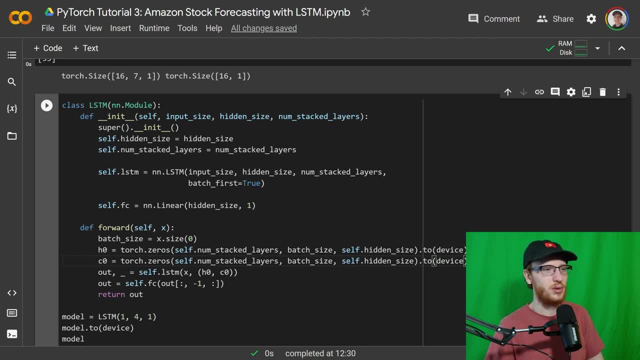 h zero and c zero things And they have to have this particular shape And they also have to be on the device that you're working on. I do not want to get into the details. it looks like this and you initialize these two things. 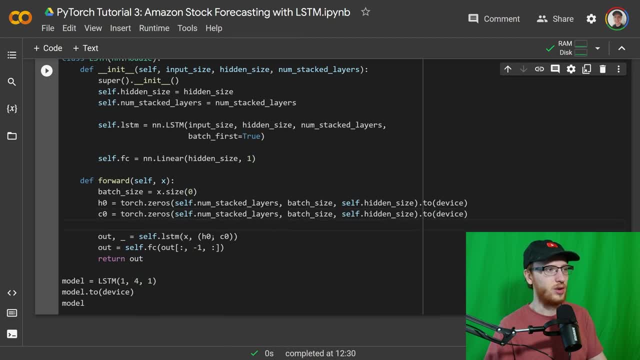 And then you're going to pass them in this tuple here when you go to use the LSTM, So you get your output that you actually care about. you get your updated tuple of your h zero and c zero, which we're going to ignore because we don't really want that Basically, after you pass x. 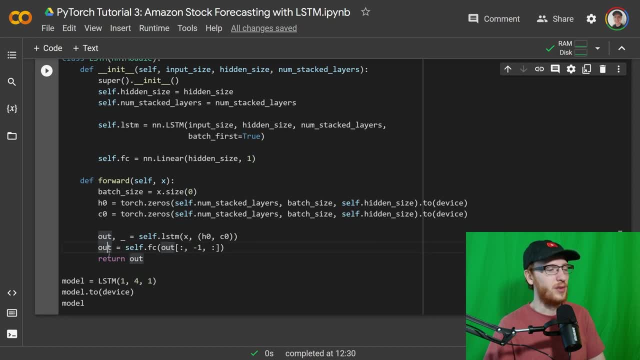 in here. it will give you your output And then, furthermore, output is not actually the output that you'd expect it is. you get output from passing in. well, of course, you have to do your test by adding a new one, but it's a new one, So you have to do a test by adding a new one. So 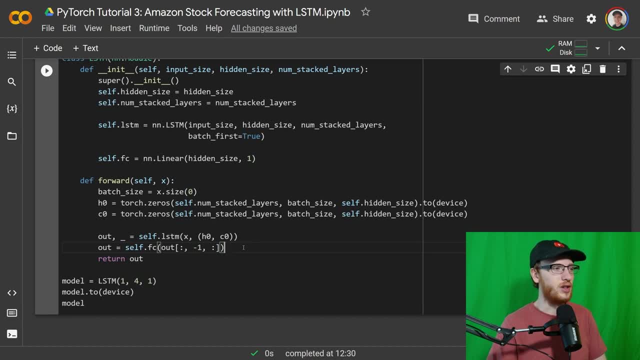 that's going to be a lot of work because we're going to pass this out: colon negative, one colon. Right now I am not digging into the details of why that is the case. trust me, it is going to work. we create a model where we're passing it. we have one feature, just the closing value for 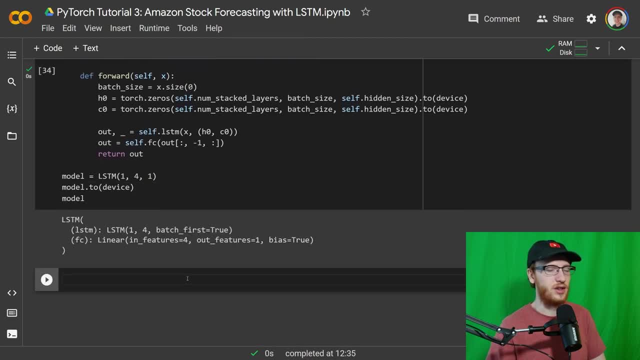 hidden size. you could play around with that If you want. numstacked layers, you could also play around with that if you want. but just one will be fine. We will create our model, put it to the device And here you go. 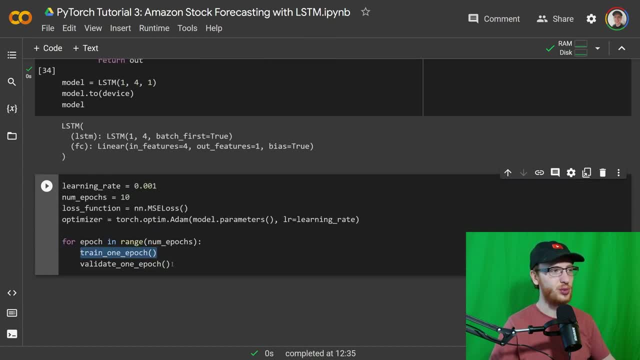 in the same format that I did in the first tutorial. I want to first show you how to do that, So I'm going to start with this and then I'm going to do this. I want to first show you the training loop using functions we haven't quite written yet for train. 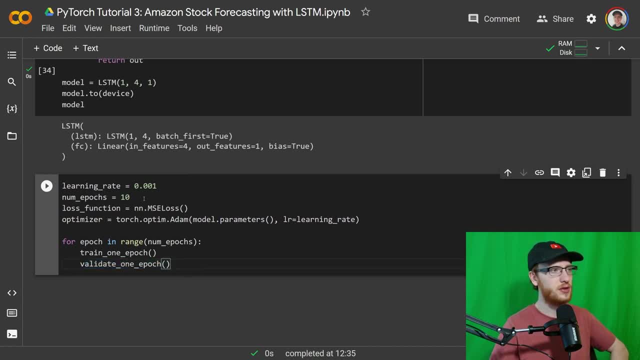 an epoch and validate an epoch, And in a moment we'll write those functions- Although I'm not going to go into them as much detail, because I covered them a lot in the first video And we played around with it a bit in the second video. So I would check those out if it's, if it's a. 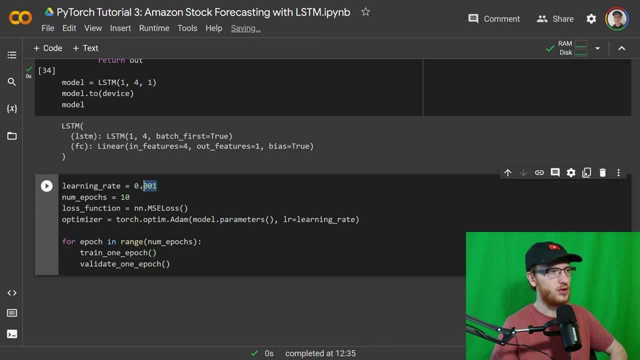 little confusing to you, But we're going to specify our learning rate. we'll start this at point 001, number of epochs. we're going to make this 10. loss function is the mean squared error. that might look a little surprising, But this is basically a form of regression problem. 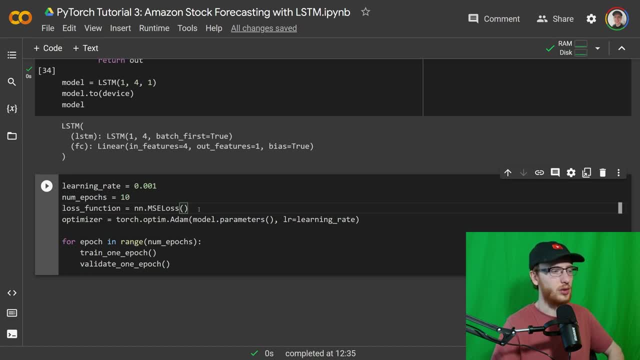 we're still predicting a continuous value, And so we are going to try and minimize the mean squared error or optimizer we're just going to use the standard atom, bypassing the model's parameters and the learning rate that we adjusted, And then, for epoch, in the range of the number of epochs. 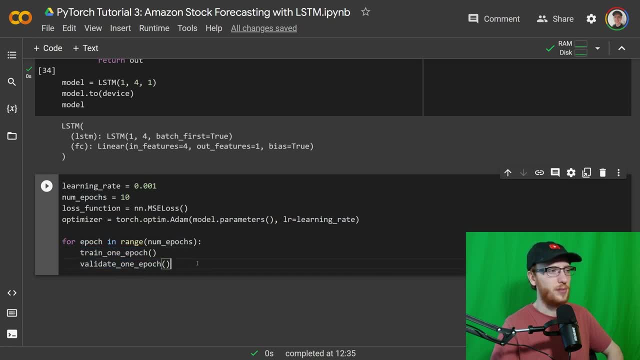 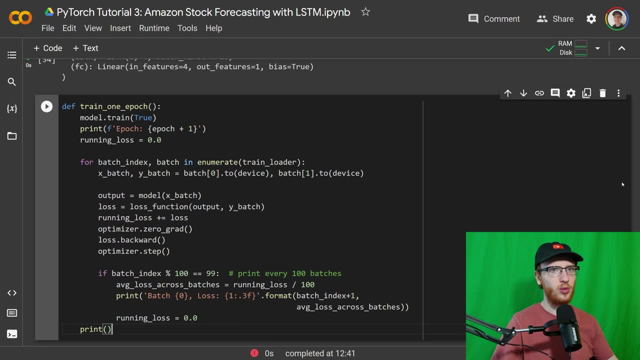 we are going to train for an epoch and validate for an epoch. Now let's write our train function. Okay, so making sure to put this above our training loop. here we have train one epoch which is going to set the model to training mode. we will print the. 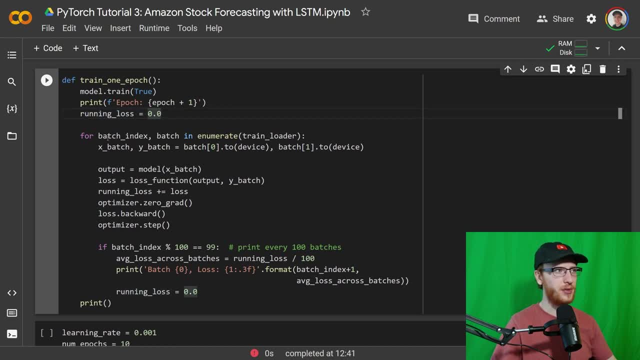 epoch and we'll start to accumulate this running loss value that we're going to loop over the train loader. So this basically just gets a batch and keeps track of the index And we'll get our x batch and our y batch from the batch and put it on the device that we're using. we will get our 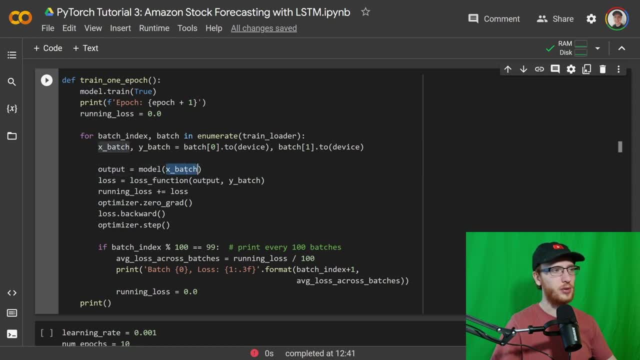 output, which is getting our output from the model. So we put in our x batch into the model that gets our output and we get our loss is the loss function of the output and comparing that to the ground truth, So comparing our models, 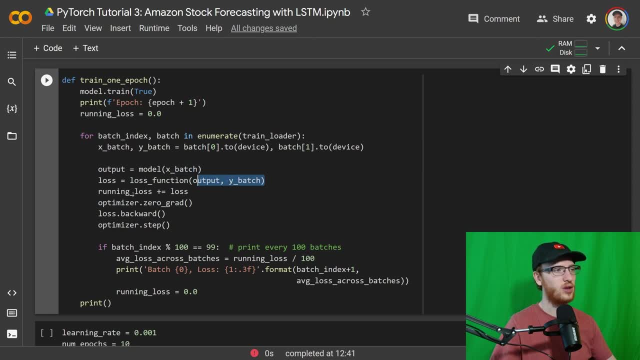 outputs to the ground. truth is our loss value. Then we get the running loss is plus equals the loss. This should really be dot item, but it doesn't really matter. Basically the loss is just a tensor with one value, And so we will get item which just actually gets the value from that. 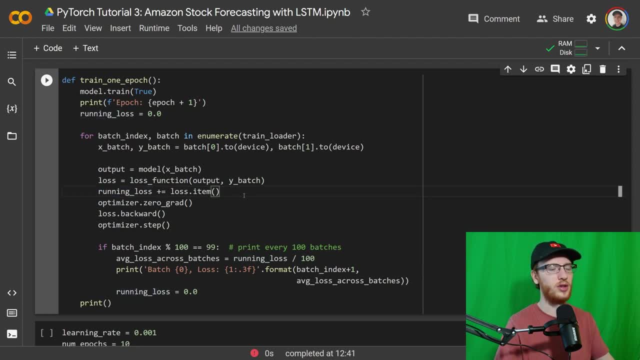 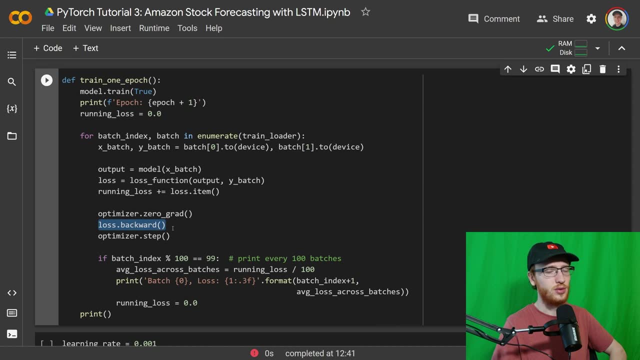 tensor. So running loss plus equals the lost item will accumulate that loss. And then we zero out the gradients. we do a batch and we get our loss, And then we get our loss, And then we zero out the backward pass through the loss to calculate the gradient, And then we take a slight step in the 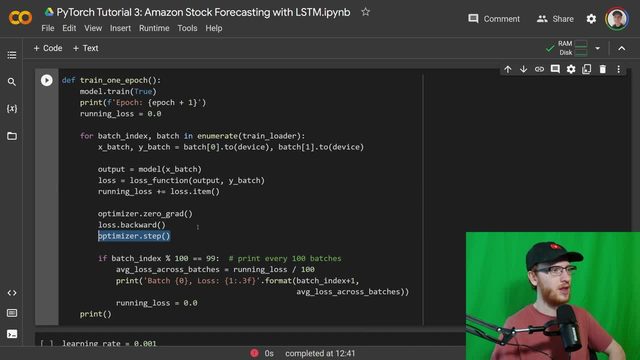 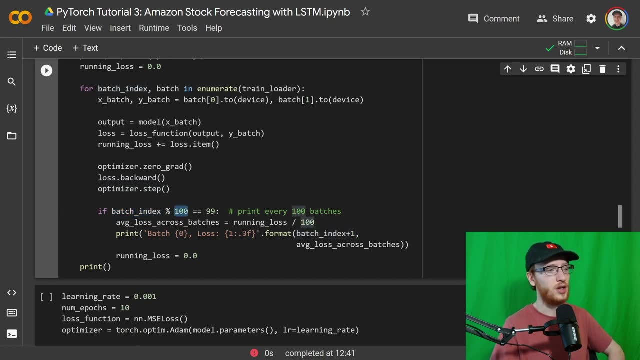 direction of the gradient, to make our model just a little bit better than every 100 batches. So this says, if the batch index mod 100 is 99. So at the 100th batch, or every 100 batches, we will get the. 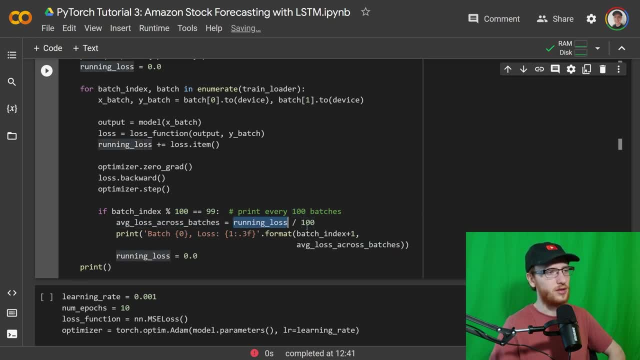 average loss across those 100 batches is the running loss divided by 100. That'd be the average, And then we print the batch and the. it should be the average loss for the batches, but we just write that as the average loss, So we'll just print that And then running loss should be reset back to. 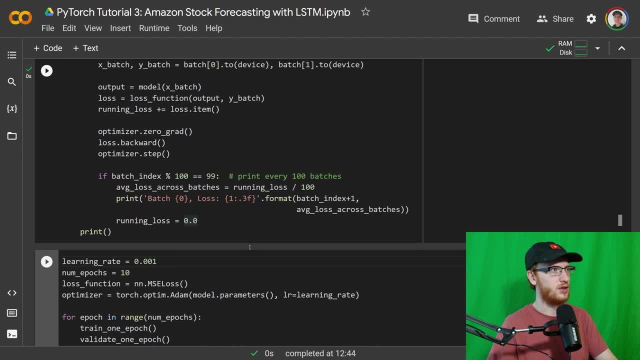 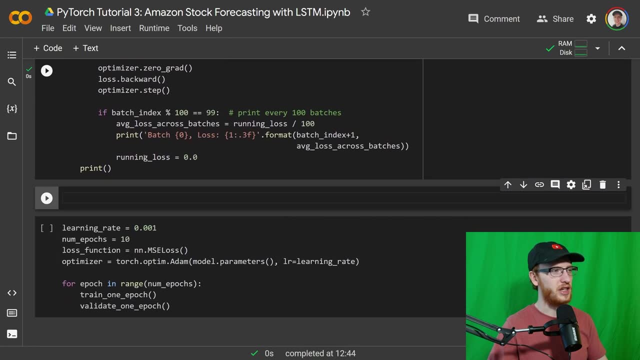 zero. So that's proper. We will execute that. just create the function. And now let's make our validate function, So putting this above our training loop again, and we'll put it below our train, although it doesn't really matter. Here we set the model train to be false, So basically put: 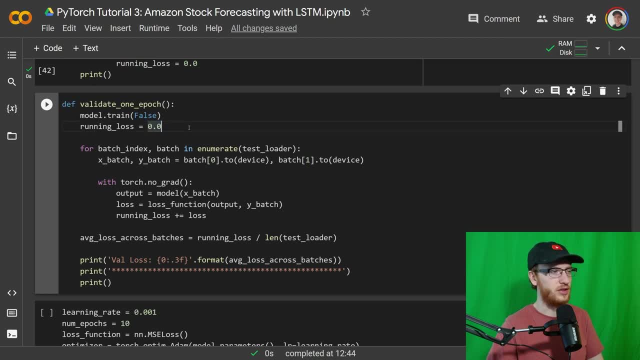 in evaluation mode we specify a running loss starts at zero And then the batch index and the batch is going to enumerate the test voter. So we're going through getting the test voter to be batches from the test voter. There's our x batch and y batch And then with no gradients, we don't. 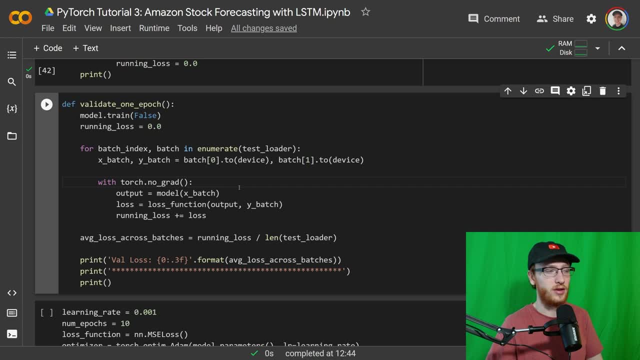 need to calculate a gradient because we are not doing any model updates So we don't need those. we get our output is just putting that x batch through the model. we accumulate our loss by sorry. we get our loss by the loss function is comparing the outputs that we got to the ground. 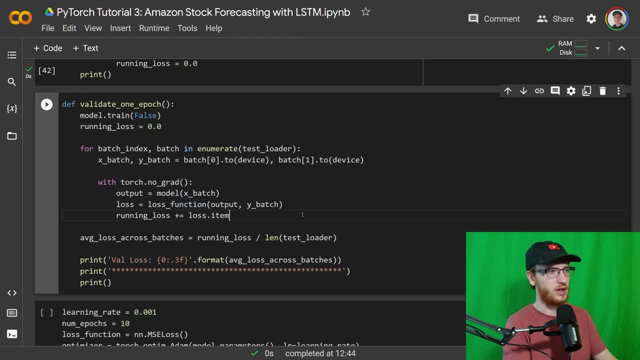 truth we accumulate our running loss by again I would make that accumulate. the loss dot item we get average loss across batches is the running loss divided by the length of the test voter. So across all the batches we get our average loss value And so we can print that down there. we will run that And then let's quickly. 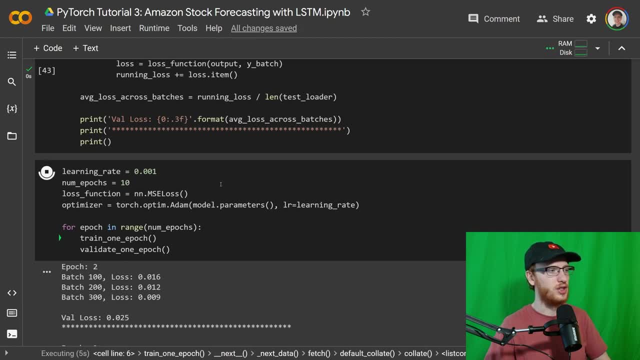 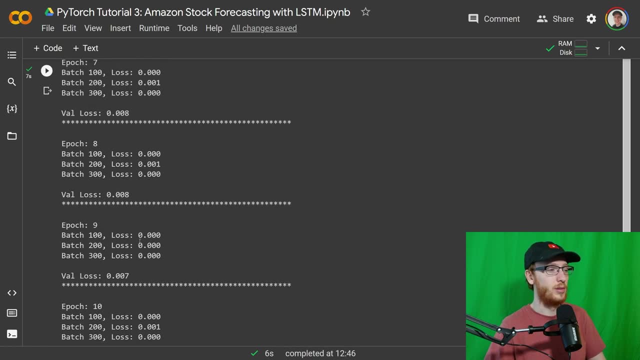 just check if this works. it is working, And we should probably train with the GPU, Although actually it's pretty fast. No, actually, okay, fine, We're sticking with CPU for this lesson Because I mean it are the model already over fit. So let's take a look So you can see the loss was. 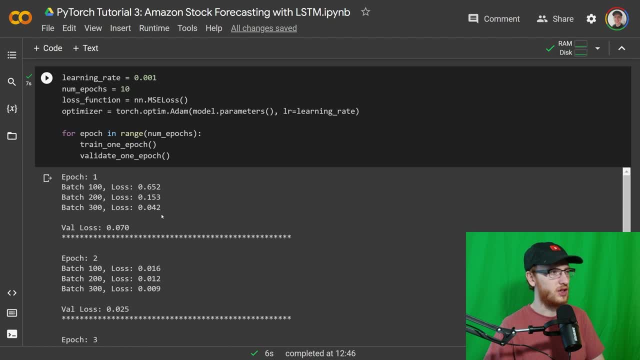 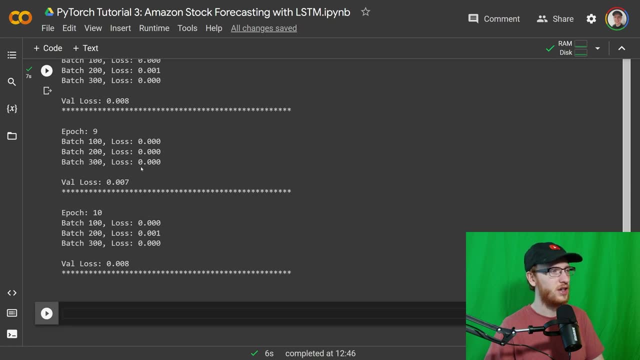 very high at first, but it very quickly figured it out. So it goes down. Validation loss goes down And yeah, this, this seemed to train just fine. it actually was perfect, And I mean it was on purpose, because I had set this to 10 epochs. If you were training your own, 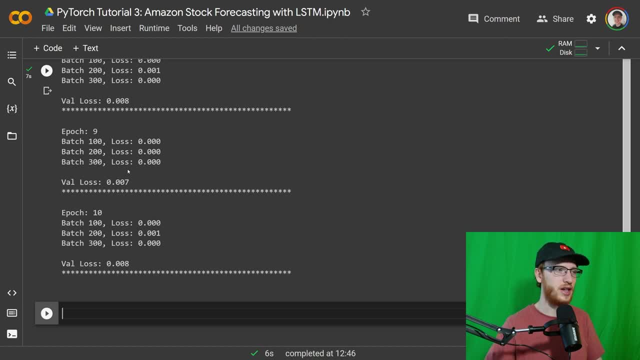 model. you would, of course, always have to play around with the learning rate, the batch size, the model architecture, But I'm setting this up so that this works right away. And yeah, let's carry on And let's look at our model. Okay, this is just some code to do, some plotting, So we're going to do. 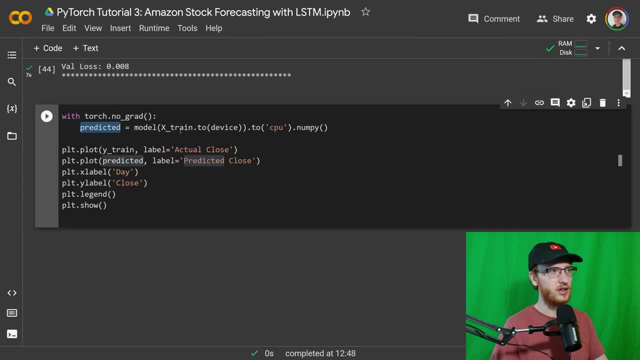 no gradients when we get our predictions, So we'll get our predicted For the x train. So this is for putting all the x train stuff in to get our predictions for the first 95% of the data. Remember, the models already seen this stuff, so it should do pretty well. But the model takes that in. make sure that it is on the device when you're putting it into the model And then you have to put it to the CPU in particular. that's not a typo, Because after you convert it to NumPy. well, NumPy doesn't use the GPU, So the stuff that you're using better be located on the CPU. 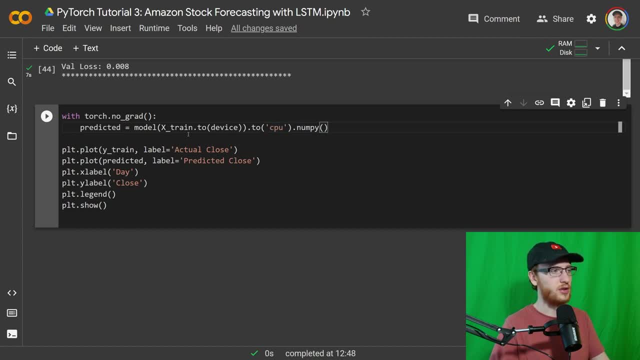 So we put it there. So we've got our predictions for the first 95% And then we do plot. we plot the y train is the actual closing compared to our predictions for that, And then we plot the day and the close and we should see our graph where the orange is depredicted And the blue is the actual. remember the models already seen this before in training, so it should be pretty good. But you see the day as it goes on And the closing value, Whoa, is a value from negative one to one. That's just main knowledge was practiced. 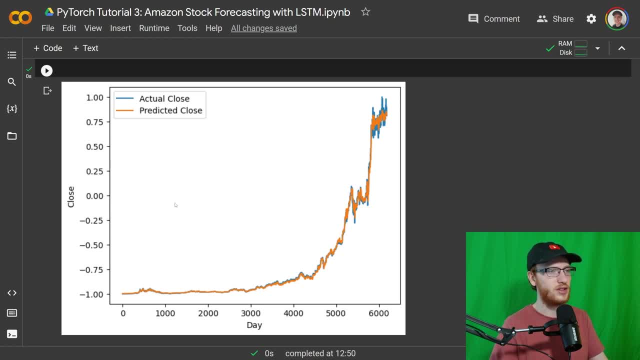 so remember, we scaled this data on purpose, so it's all in this small range for the network to use. but we're definitely going to have to use an inverse transform in a moment because we don't want to look at these values. it just looks weird. now this next piece might be a little confusing. 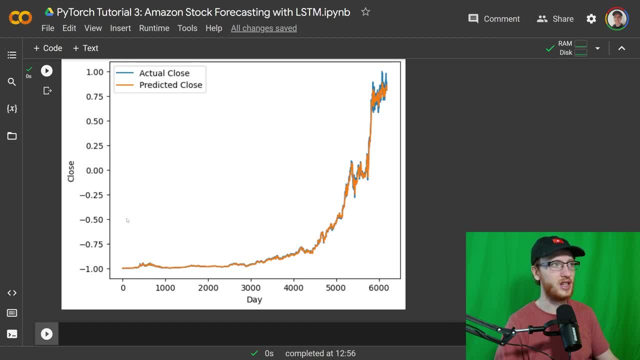 but i'm going to take it really carefully. here we have our values between negative one and one, so we need to do the opposite of what our transform did, so that we get our original scale back, the real numbers or dollar values that are actually useful to us. now it's not too bad, but there's a 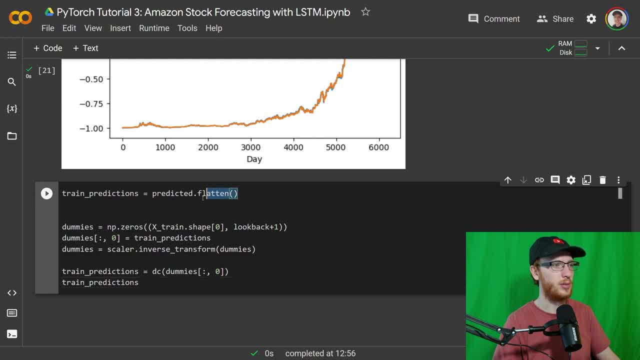 little bit of a trick that we use now. train predictions is going to be predicted dot flatten. that's not a trick, i just making sure that it's one axis that's important. and then dummies- why do i? what am i calling this dummies? well, it's a zeros matrix and we'll look at it in a moment. 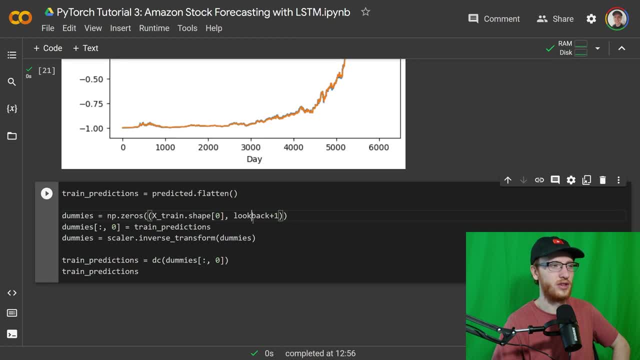 but basically i don't care about what most of this stuff looks like, it's really just having the proper shape, and then we're going to adjust. the first column, so, dummies, is the zeros, where it's the shape of the x-train shapes of zero. so the number of examples that we 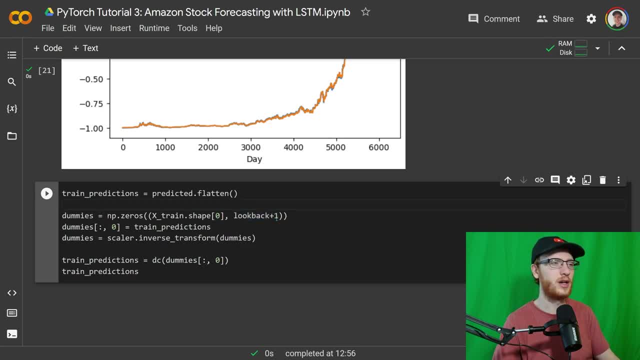 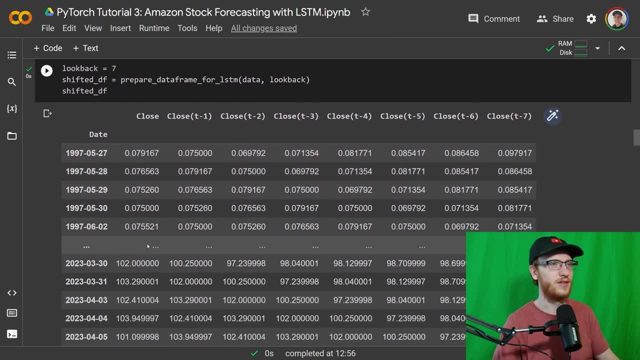 have here and then we're going to adjust the first column. so, dummies, is the zeros where it's, and then our look back plus one. it's look back plus one, because that is the length of this whole thing. okay, so i'm trying to make a dummy matrix that looks like this: so look back plus one. well, 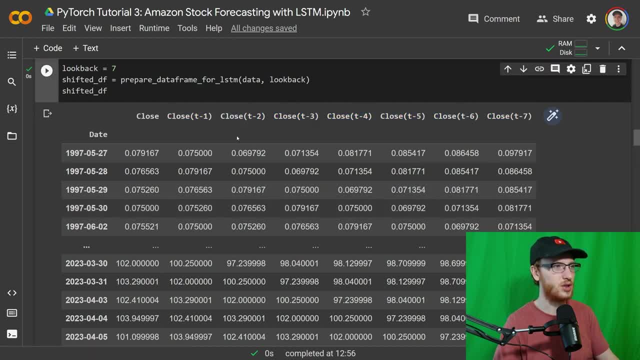 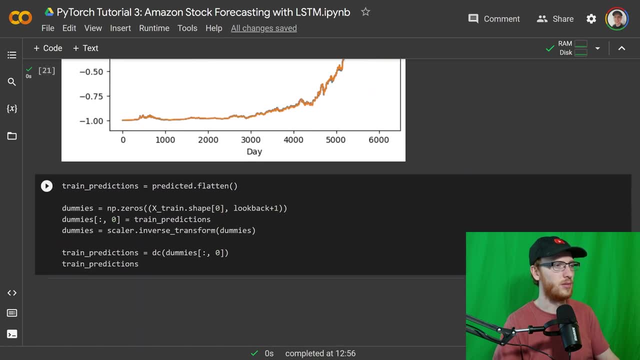 this is seven, so look back, what plus one should be eight. so it's the same length here, and then it's going to be the row wise, the number, uh, that we have in x-train. so why am i making this weird dummy matrix? well, it's so that i'll set the first column, this sets the first column, and then i'll. 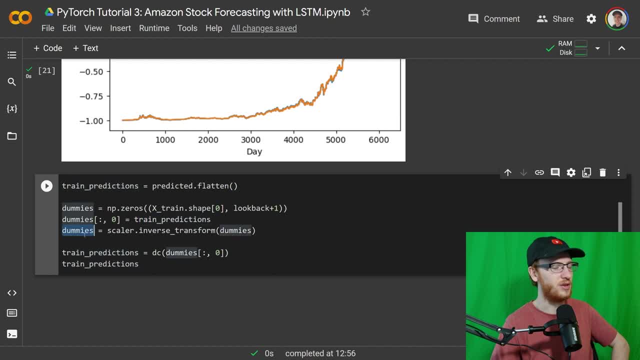 set the second column of that to the predictions that we have and then we can apply our inverse transform, because our transform is used to taking that whole matrix and maybe i don't know if you guys know an easier way to do this. maybe there is, but basically i just made a matrix that has the 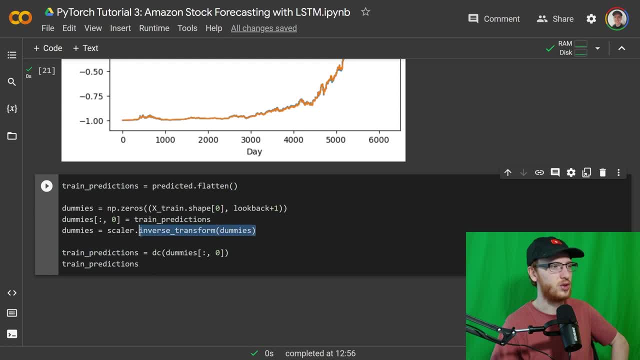 same shape as what the scaler was used to. and then i did an inverse transform on that whole thing so that we can again just care about the first column. so it actually transformed that first column. well, and then we'll get back our train predictions in the right scale, and then we'll 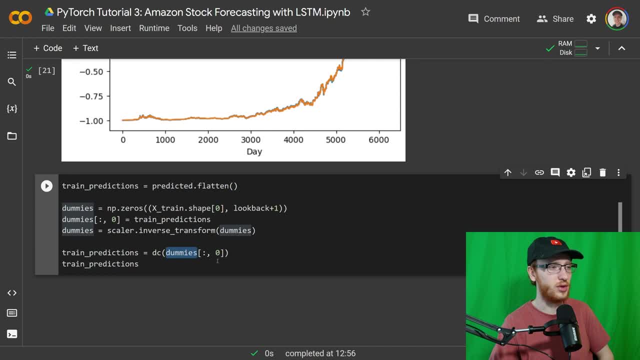 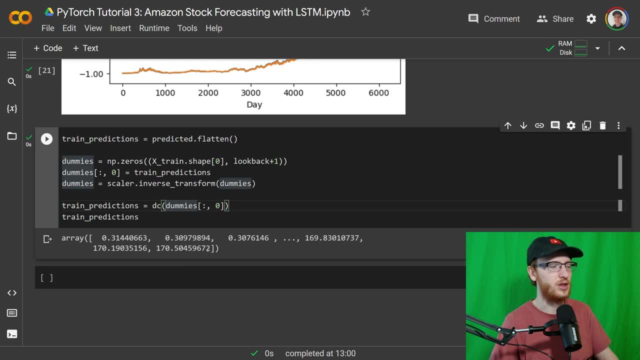 get our dummies is we're going to get a deep copy of that dummy's first column again. that transformed column and train predictions is only that first column that i'm selecting and here you go. you should see, early values should be very small numbers, like we saw, and high numbers should. 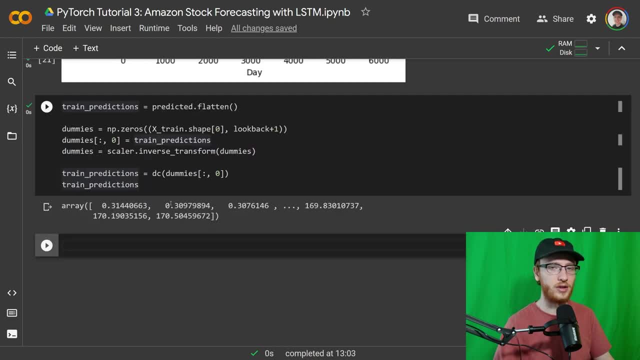 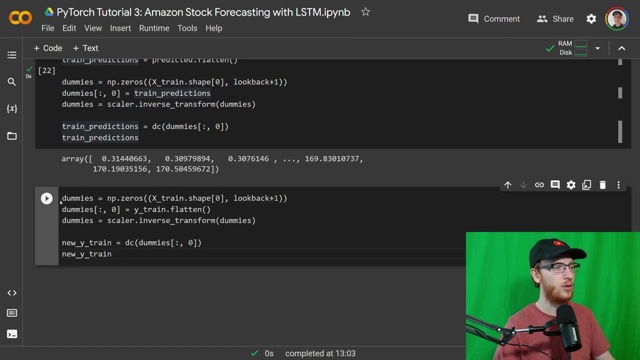 be or later. numbers should be high numbers, like we saw. now we're going to do something very, very similar for the ground truth. this was for the predictions, but now for y-train, since that's also currently on the wrong scale. we get our dummies is our matrix. that looks basically the 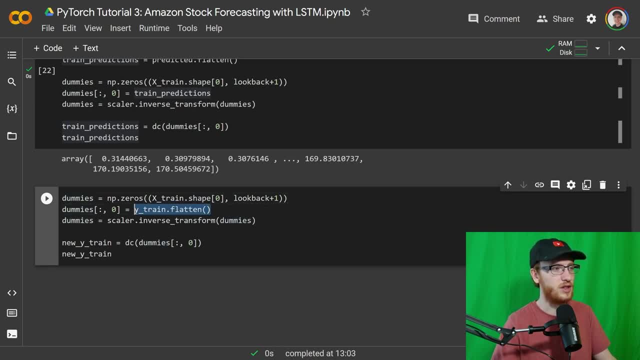 same thing, dummies, is that first column is now going to be y-train dot flatten. so we update that first column, apply the transform on that whole thing and then we get new y-train. it's just going to be a deep copy of that updated first column and we should see y-train there. now we're just 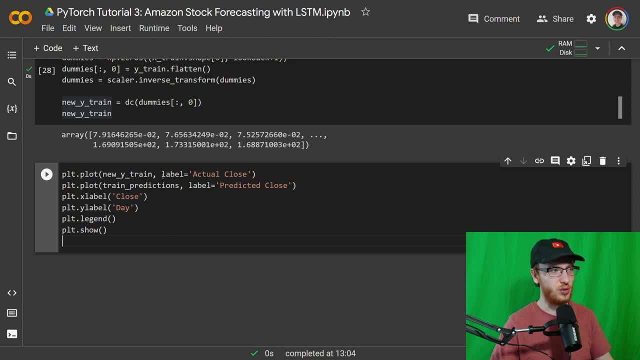 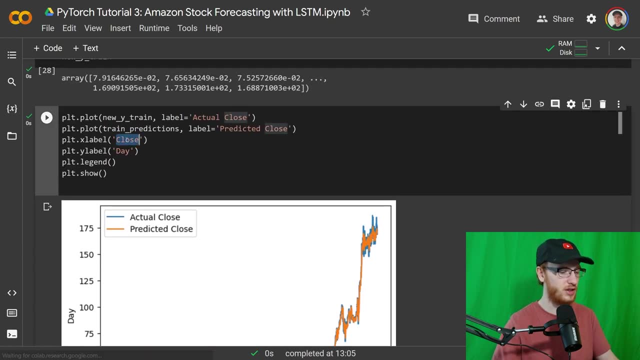 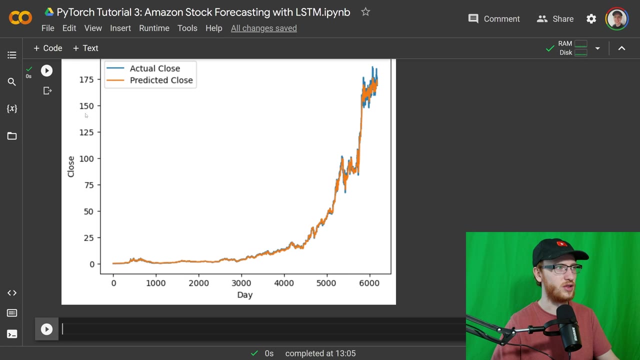 going to make the same graph. it's exactly the same thing, except we have new y-train there and train predictions should be the same as before. looking at the close: oh sorry, those are backwards labels. this should be day and that should be close. so here you should see the day on the x-axis close on the y-axis before, except now. 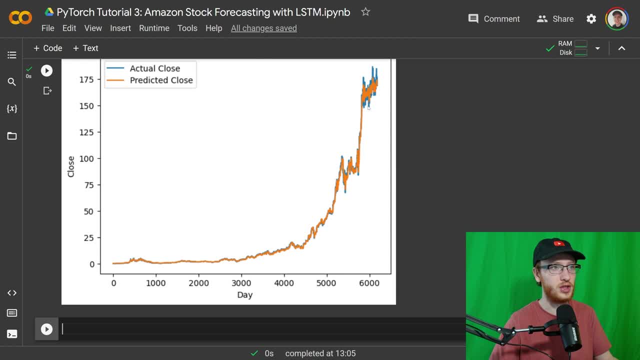 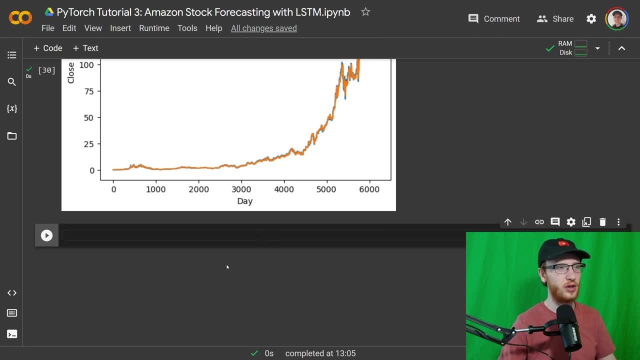 they're on the proper scale. so the graphs: they shouldn't really change or look any different, it's just that they're on the proper scale now. now we need to do this for our test stuff now. i'm going to do this all in one chunk here. before, we kind of looked at this intermediate graph, which 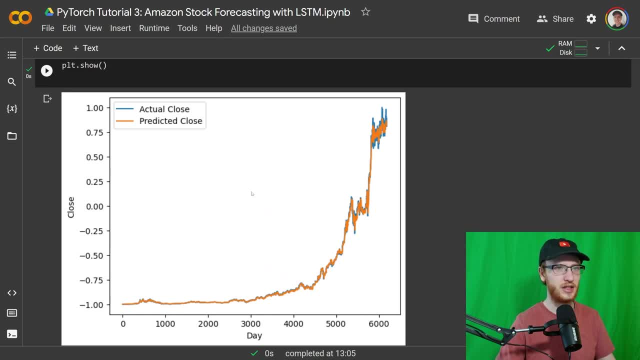 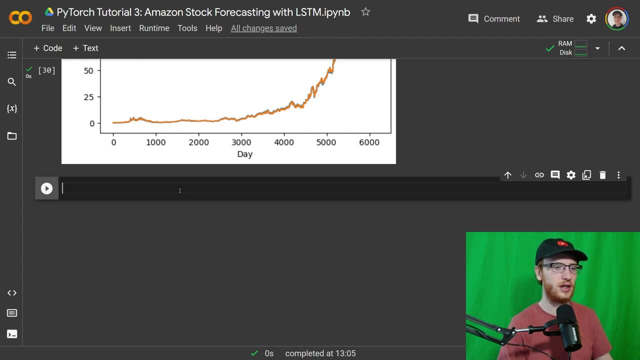 was we had on the wrong scale. i'm just going to show you how to get the test predictions and convert them to their proper scale here, and i'm purposely using slightly different code just for pytorch to get different practice with different functions that do similar things. that's a lot of. 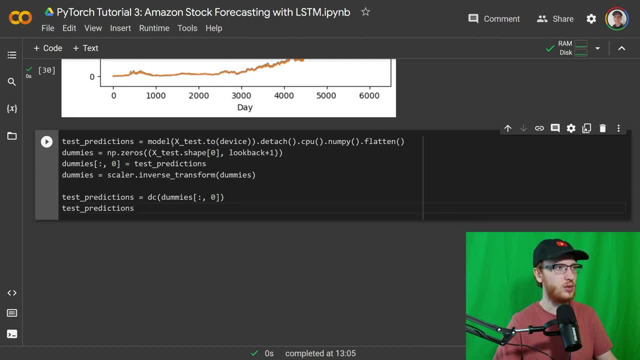 wording, but just take a look. so test predictions is: you again get your x test and you put that to the device, the model's on, you get our outputs. then we do dot detach and you'll notice- oops, not that you'll notice- there's no torch dot, no grad here. this is kind of an alternative in this. 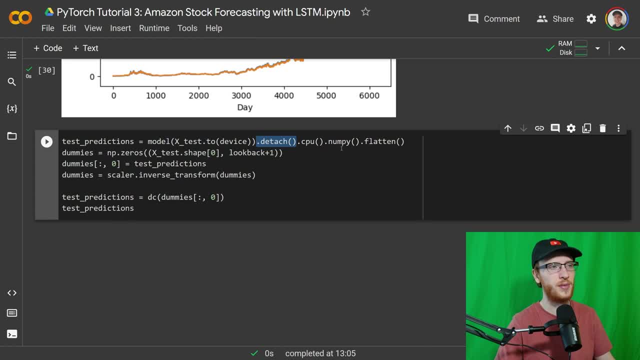 situation where we detach this from the computational graph, then we put it on the cpu, then we can do numpy and we're going to flatten that as well. so it's a very long chain of these things and that's not, unfortunately, not uncommon in pytorch, but it gets the job done. basically it is just a vector of our test predictions. if you're using 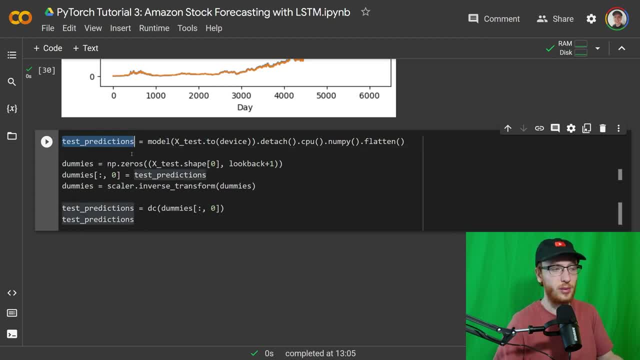 tensorflow. it genuinely would just be like you just run them through the model. but that's what it is. dummies is the same thing as before, so i'm really not going to explain that. we are just going to convert our test predictions to the right scale and we'll run that and you should see the proper. 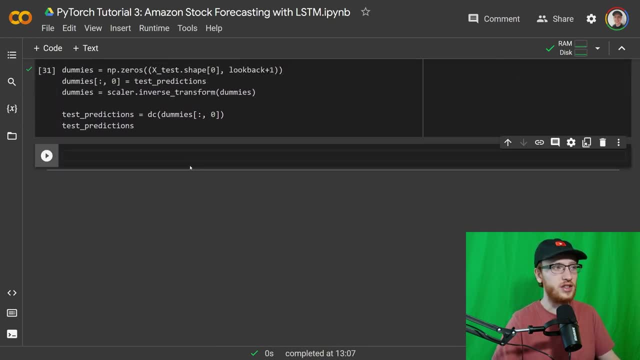 scale on the test predictions. there we need to get our ground truth on the proper scale. but this time it's for y test. i don't want to explain this because it's basically the same as it was for y train and now we have new y test on. 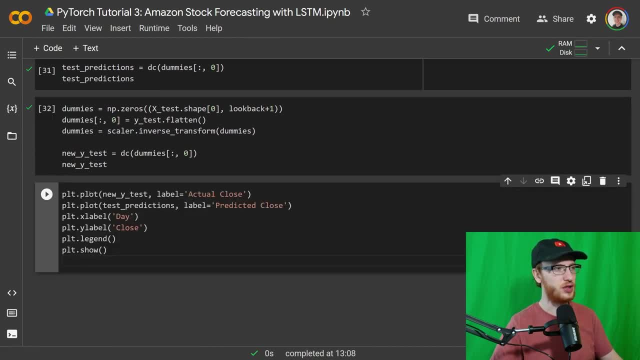 the new scale and let's just finish this off with our final graph. so this should be our new y test, our ground truth that the model kind of seen like it hasn't actually seen it, it just evaluated through it, and our test predictions as well. so on the proper scale, we have our actual and our 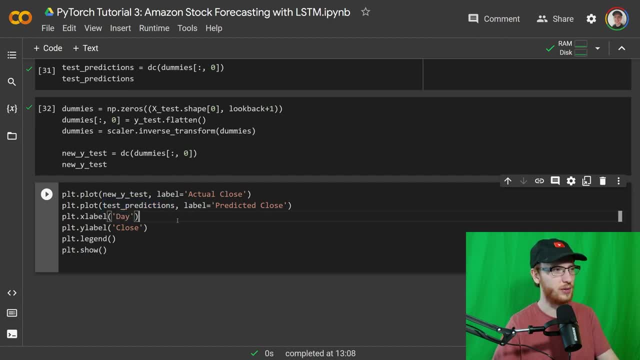 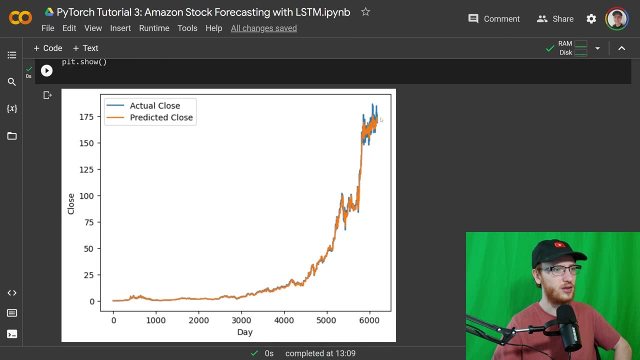 predictions we have. this is probably okay. this is the right labels, time, day and close, and here you go. okay, so after this is the part that occurs after this piece. here you could optionally do some extra work to get what these particular days are, although it's a. 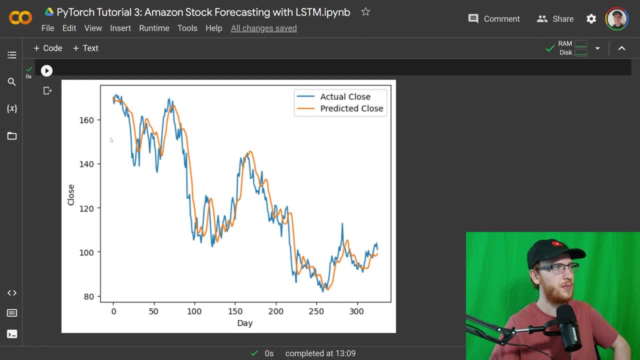 little bit annoying so i'm not going to bother doing that. good practice if you want to. this is what the model did, so you can see it's kind of just lagged behind it. it's following it pretty, pretty well. it's hard to do forecasting well, like stock forecasting. if you were to actually get a. 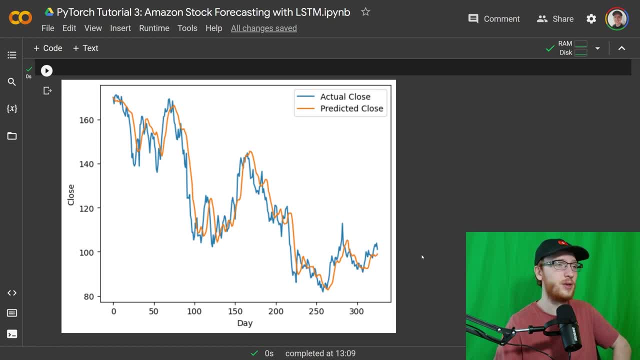 really good job of this, then, uh, then you should go to wall street. then you should go to wall street. to be honest, that's uncommon, and uh, what you should not do is think that the model that we just created is for predicting stocks the next day. you will almost certainly lose money if you do that. 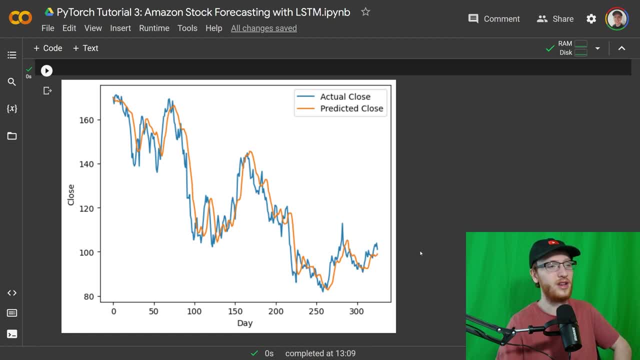 and if you even make a more complex model, of course people do it. it is kind of crazy, though. most importantly, if you are doing stock forecasting, think about the intrinsic value of a company, think about the current state of the economy. if there's a lot of negative news and 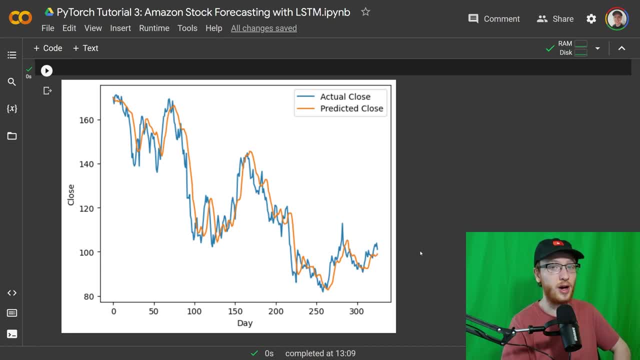 it's been down a lot recently. actually, it's going to go down a lot more than it's going to go down, to go opposite most likely, and that would be a time for it to go up. conversely, if it's been going up for a long time, it's probably just going to go down and and most of these stocks work well. 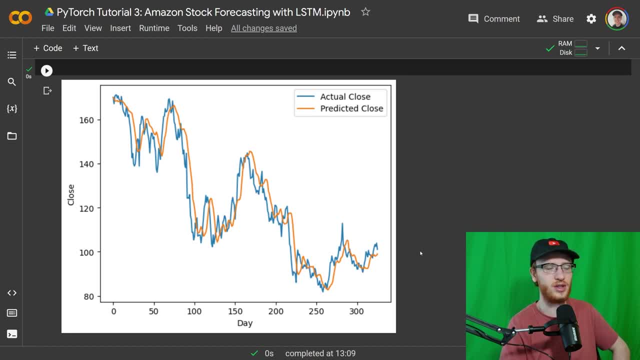 together. occasionally companies have fallouts and they have issues, but for the most part, if amazon's doing well, so is netflix, facebook, google, apple. all of them kind of work well together. so that's the sort of sort of stock analysis you should do. nonetheless, here is our lstm stock.